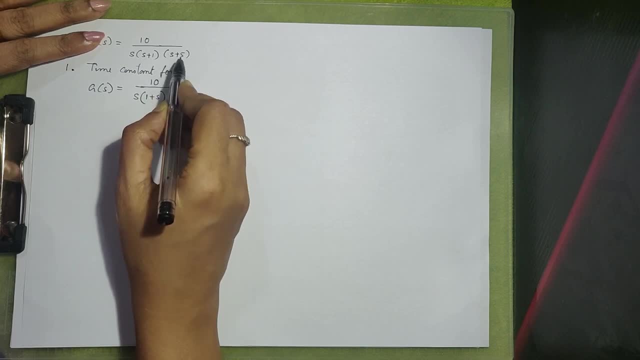 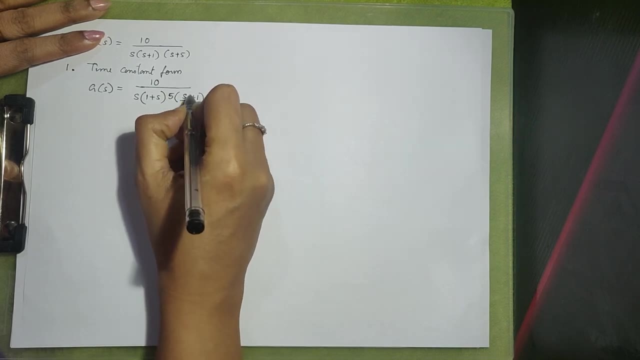 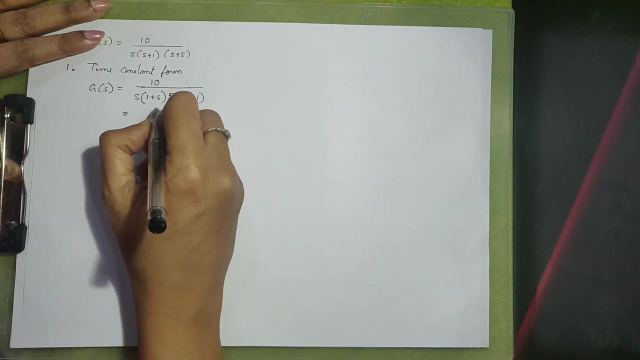 1. Then only it will be 1 plus st form. So what we will do, we will take 5 outside common, So 5 into s by 5 plus 1. So when you multiply we will be getting s plus 5 there. So this one I can rewrite it as 2 by s into 1 plus. 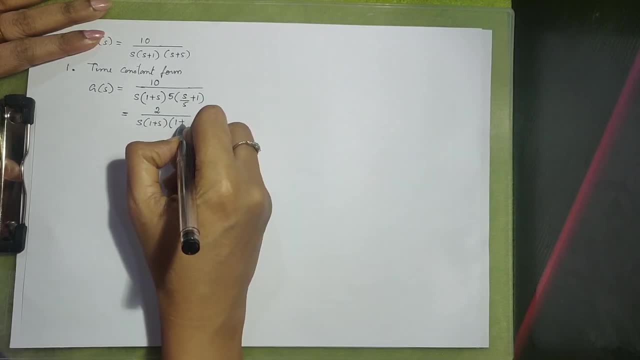 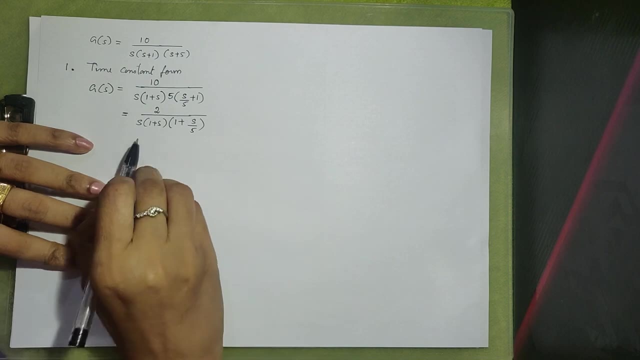 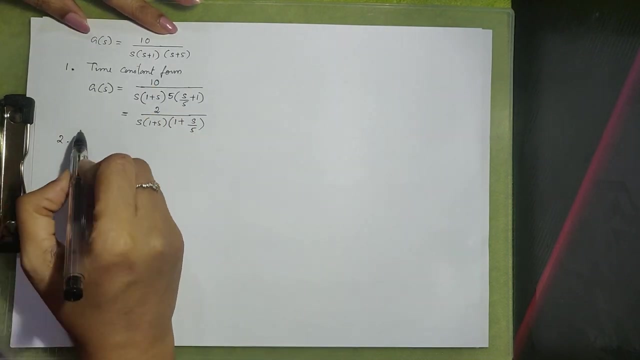 s into 1 plus s by 5.. So now we got the transfer function in time constant form. All terms are in time constant form. Now second step: since Bode plot is a frequency domain analysis we need to substitute s is equal to j omega, So suppose we have to convert this into: 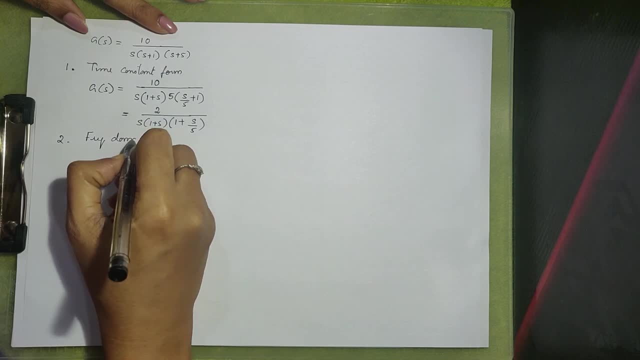 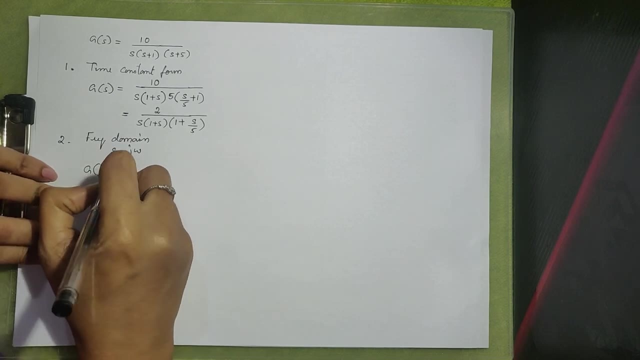 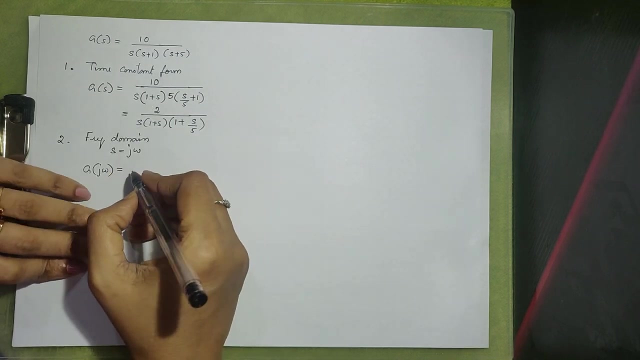 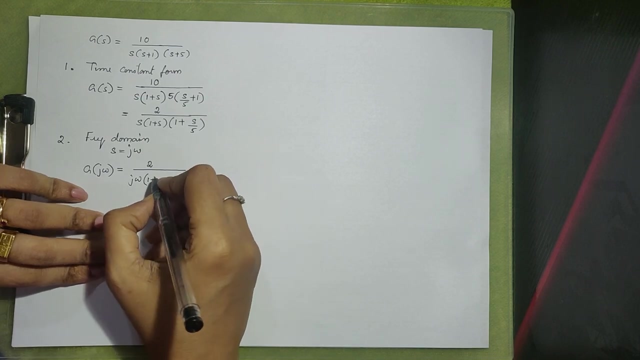 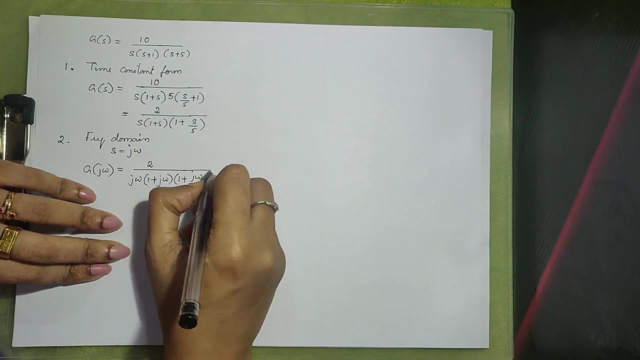 frequency domain. Frequency domain. So by substituting, s is equal to j omega. So our transfer function now becomes g. j omega is equal to substitute. s is equal to j omega, in this time constant form of the transfer function. So we will be getting 2 by j omega into 1 plus j omega, into 1 plus j omega by 5. So you got the. 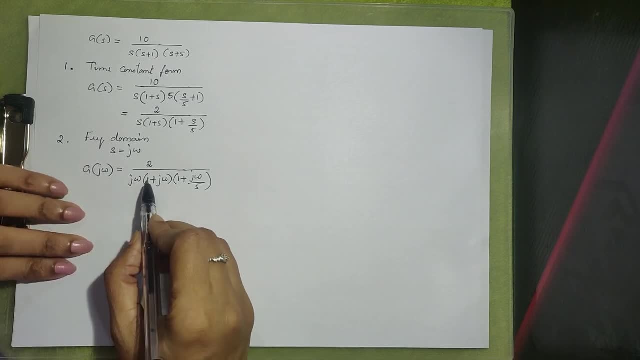 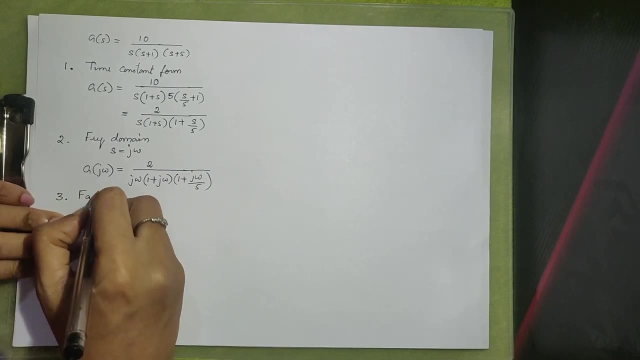 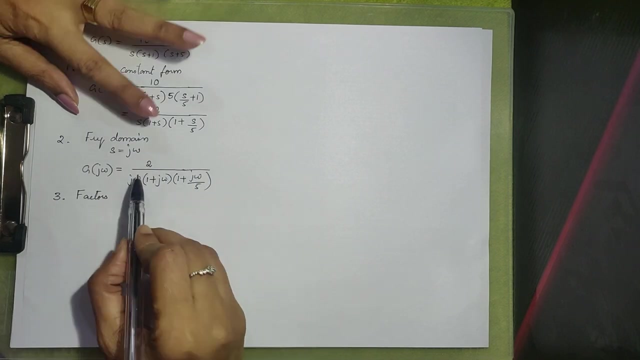 transfer function, here Now in frequency domain. next step, third one, we have to identify the factors Now, factors from the transfer function. So when we observe this transfer function, what are the factors present in this transfer function? First factor is this gain, So gain. 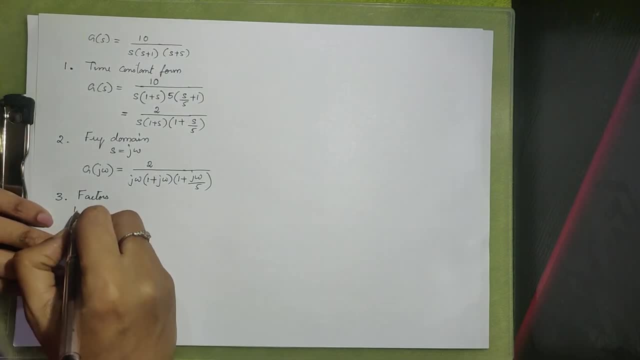 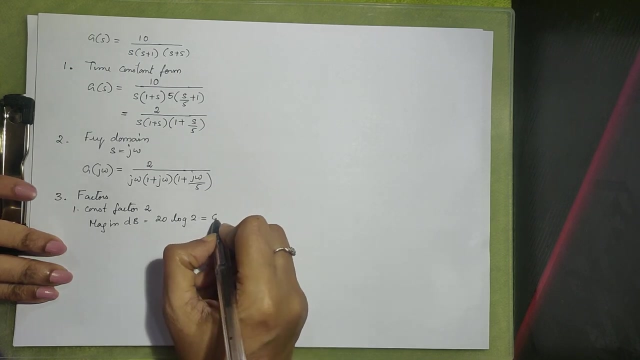 factor, that is a constant factor, 2.. So the first one is constant factor or gain factor 2.. So magnitude of this one in dB is magnitude in db for this term is 20 log k. k is 2.. 20log2.. So we will be getting the answer is 16 sub 1.. 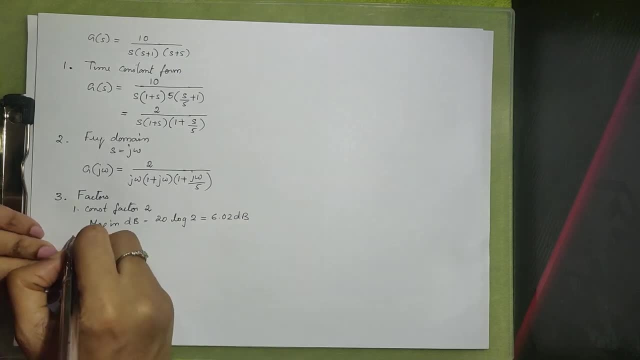 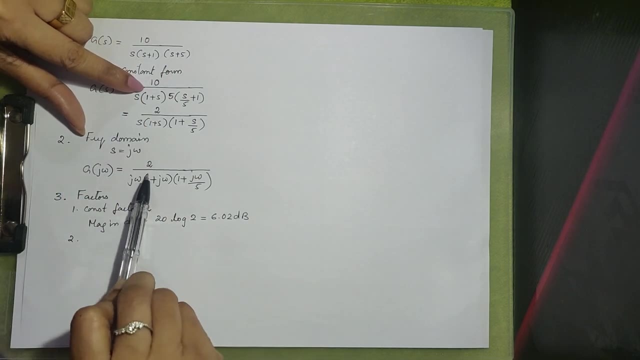 0.02 dB. Now, second term, we can see there is a pole at origin here, pole at origin present here. then we have a 0, we have 2 poles, 3 poles. we do not have a 0 for this transfer function. we have. 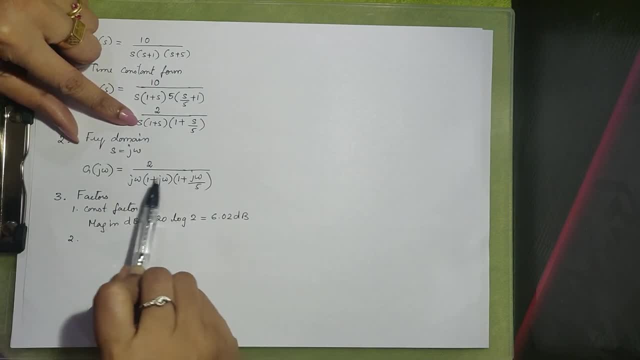 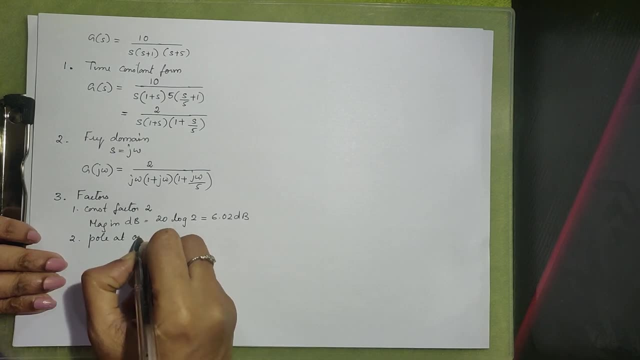 pole at origin, or we have here 2 more factors there. So the second factor is pole at origin, so which is represented by 1 by J omega term in this transfer function. The third is first order pole. so you have first order pole, first order pole, that is 1 by 1 plus J omega. we have to see each factor separately. 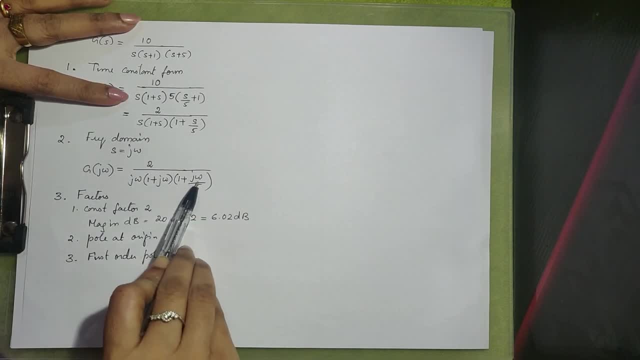 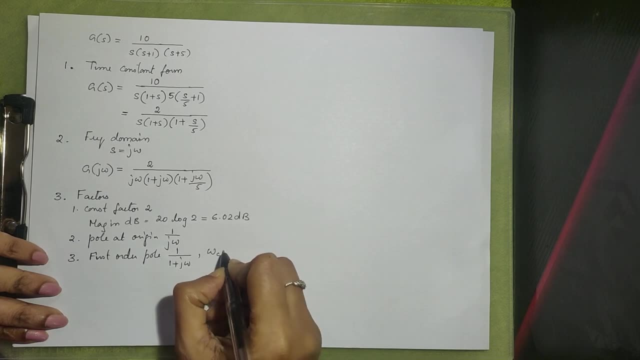 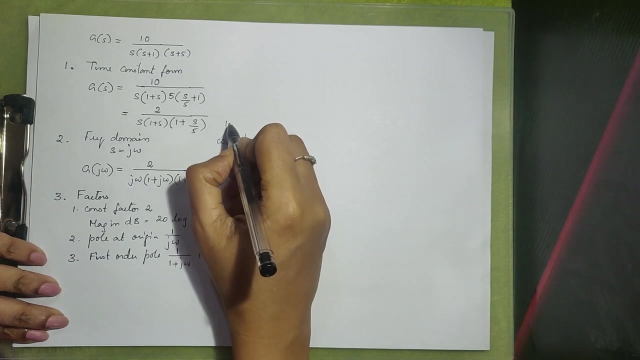 so constant. then J omega 1 plus J omega, then 1 plus J omega 5 by 5, so this one 1 by 1 plus J omega. So what is the corner frequency corresponding to this Corner frequency is nothing but omega. c is 1 by t of. if our transfer factor is of the form 1 plus st Corner frequency. 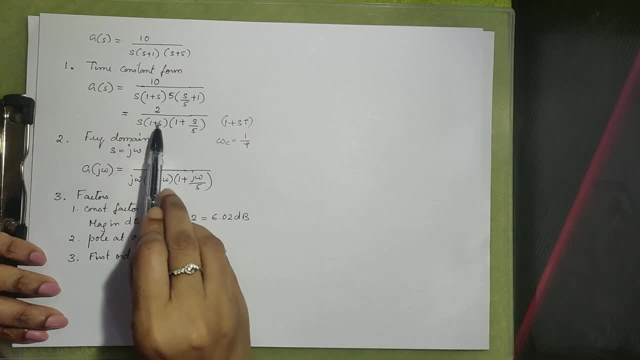 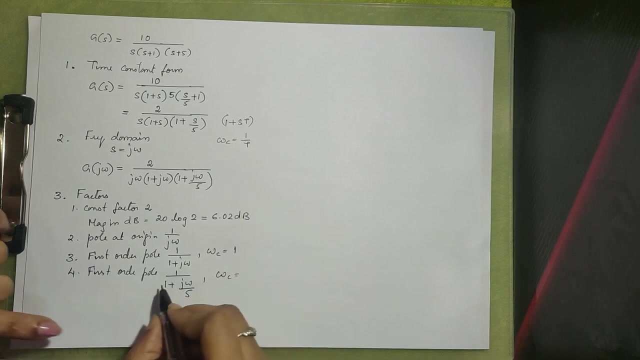 is 1 by t, So this is 1 plus st form. So here for the first term order, first term. here the corner frequency is 1.. Now fourth one first order pole again, and the factor is 1 by 1 plus j, omega by 5.. So here corner frequency is: this is 1 plus. 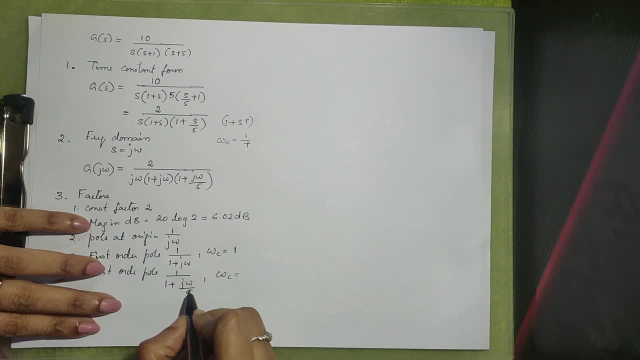 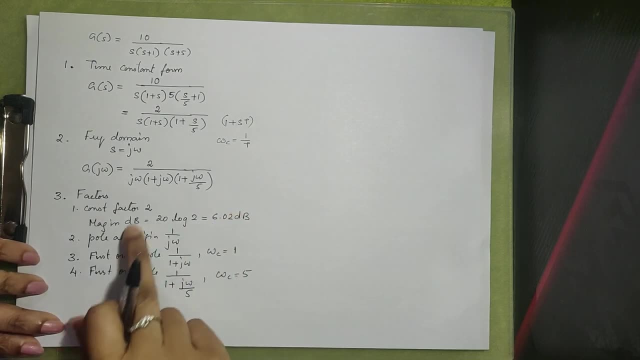 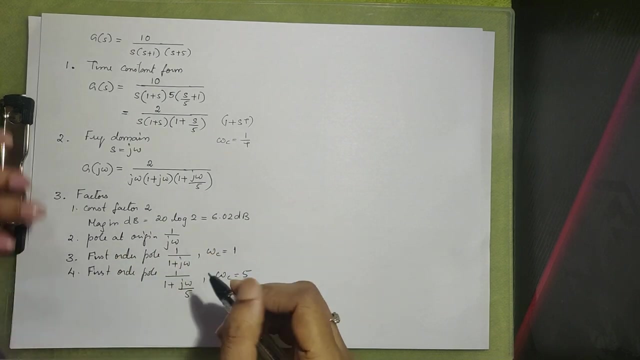 st form. So t is 1 by 5.. So omega c is 5.. So we have taken all the factors written here. Now the next step is we need to form the tabular column for plotting Bode plot. This is a main 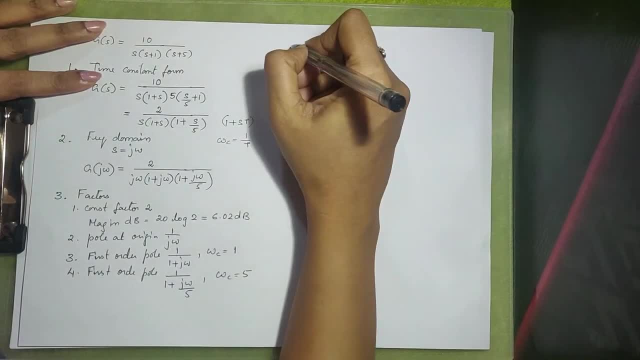 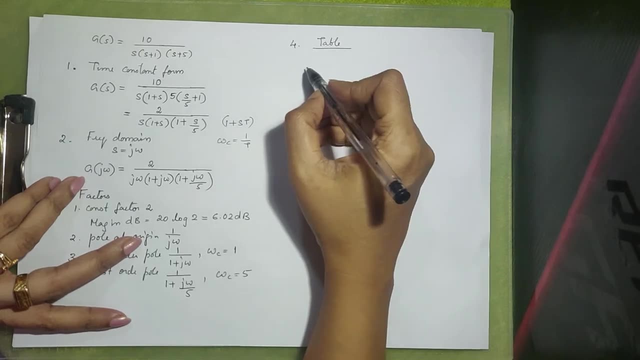 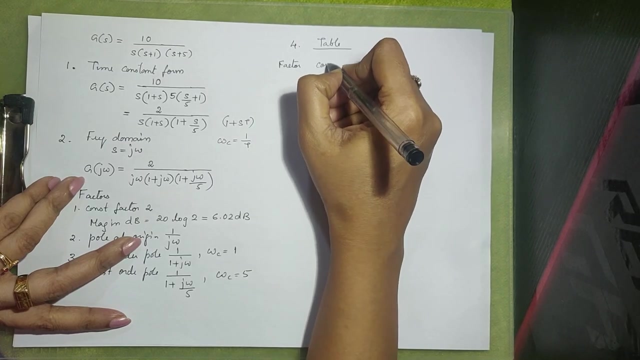 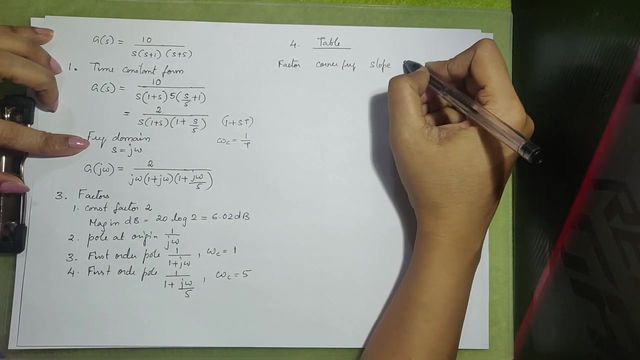 important. So we will be forming 3, 4.. Fourth one: we will be forming the table to draw the Bode plot. So here, first one, let me the first column, let it be factor, Then I am writing it as corner frequency, Then I will be writing slope corresponding to the term Then resultant. 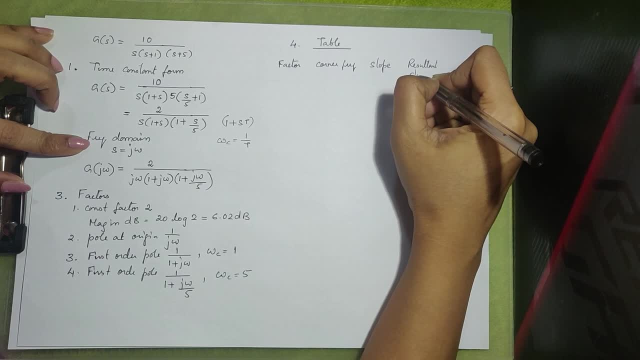 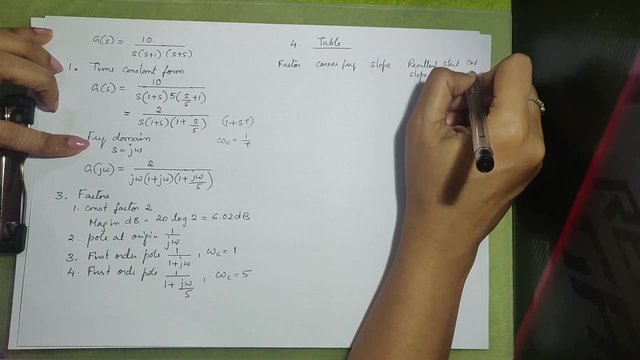 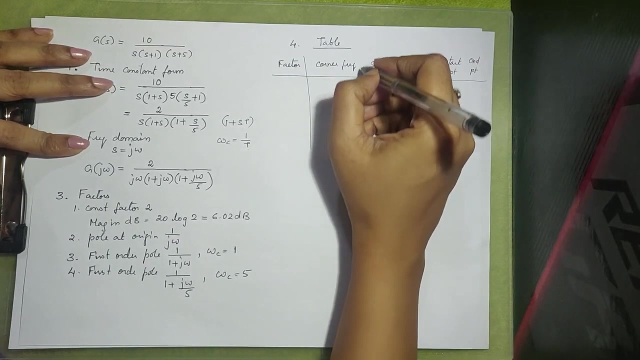 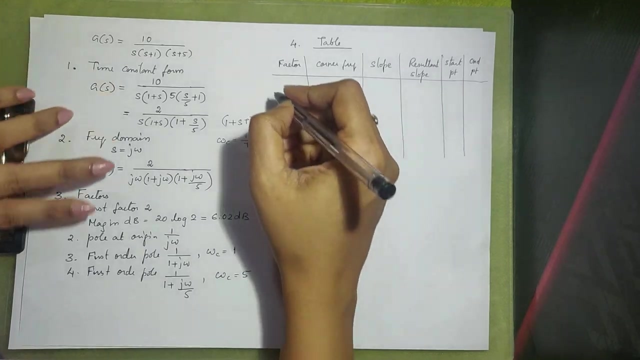 slope, resultant slope. Then maybe I can write here start point, start point and end point. So this is the table which we are going to make: factor, Then corner: frequency slope, resultant slope. then start point, end point. So the first factor here. So whenever you are forming, 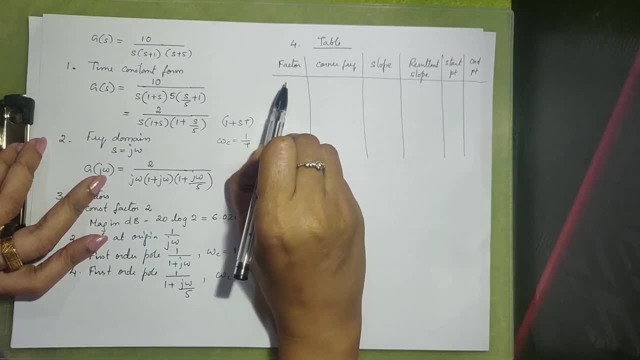 the table. you should remember that the first factor should be always B. So if we are taking the first terms, This is the first one. So here we are making 1 by 1 plus t. Corner frequency is 2 by 1 plus j. omega by 5.. So the second sec We will be forming the table. then we have 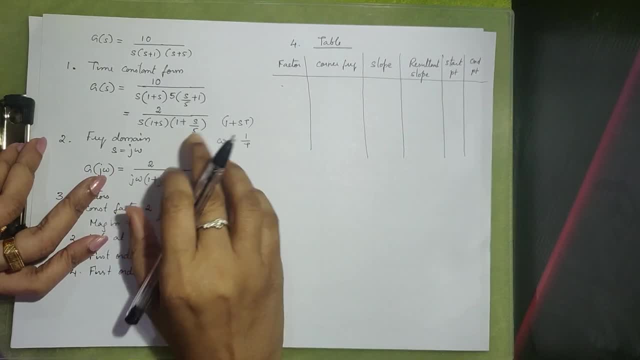 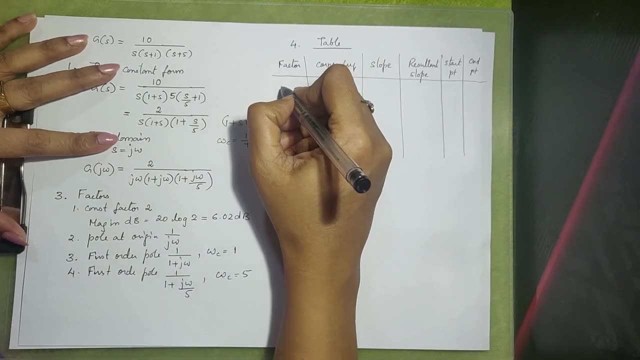 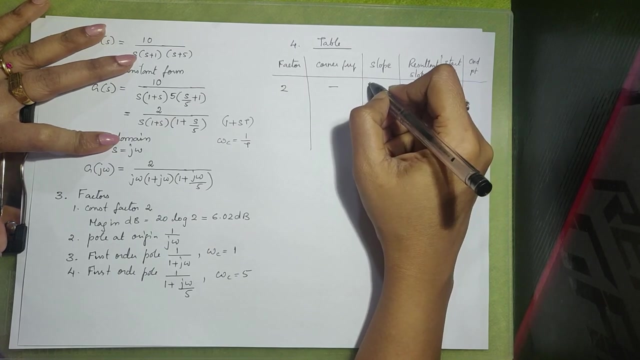 the gain present in the transfer function. if gain is not present, you need not write that. so if gain is present, that will be the first factor. so here which one is the first factor. it is two. it's the first factor. there is no corner frequency for this factor and this one. actually, here there is. 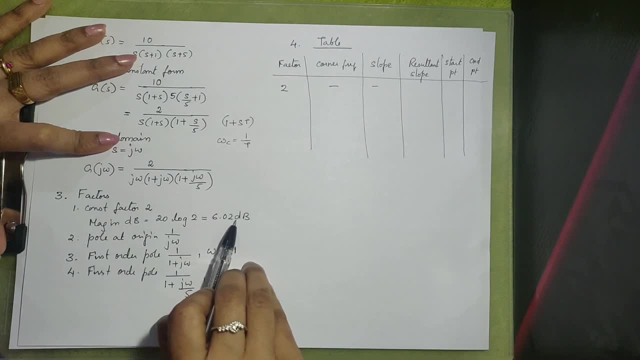 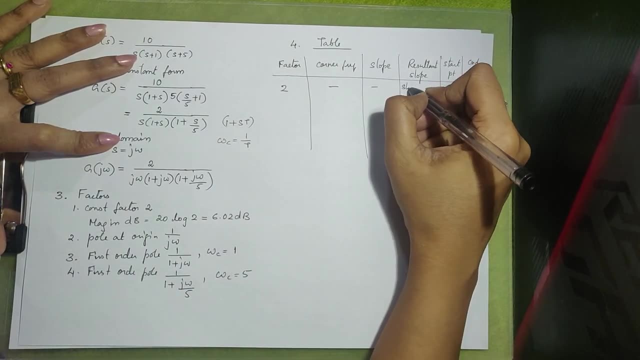 no slope for this one because it is constant log 6.02 db. so this is the magnitude, means it is a straight line, doesn't have slope. so actually it is a straight line at 6.02 db. so the magnitude it it is above that zero. the magnitude is 6.02 db. it is a straight. 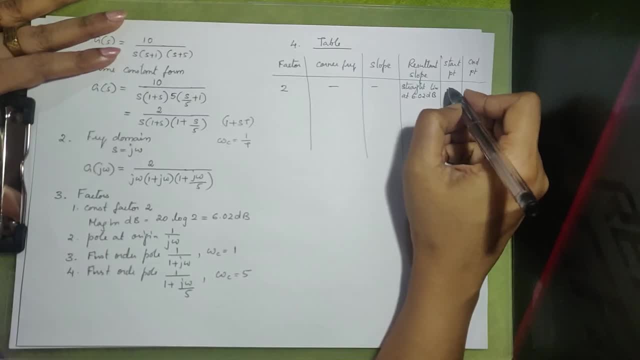 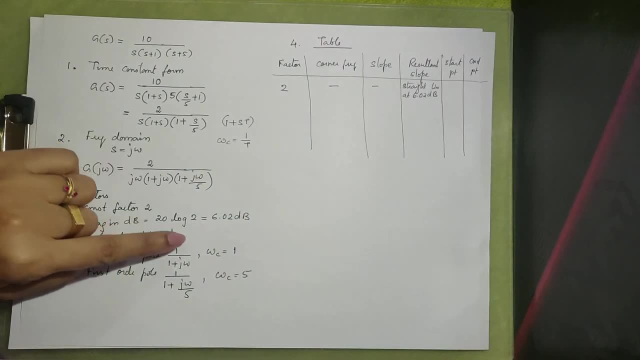 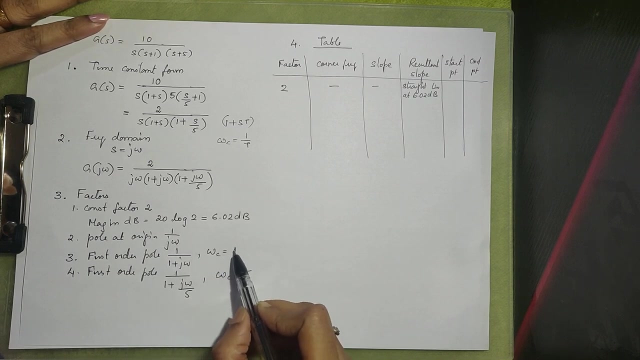 line means it is constant throughout all the frequencies. so your start point actually when you are seeing first, before finding that start point, you just have a look at the corner frequencies present in the given example. so here corner frequency is the least corner frequency you can see. here is 1. 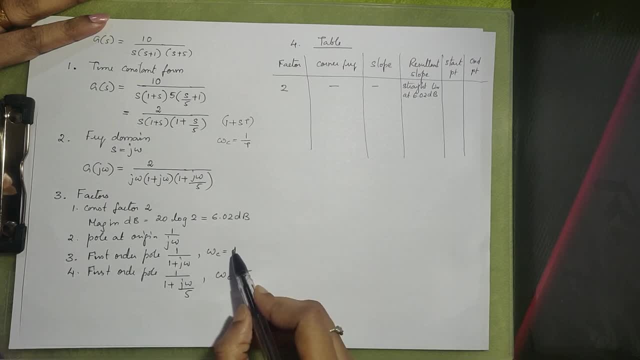 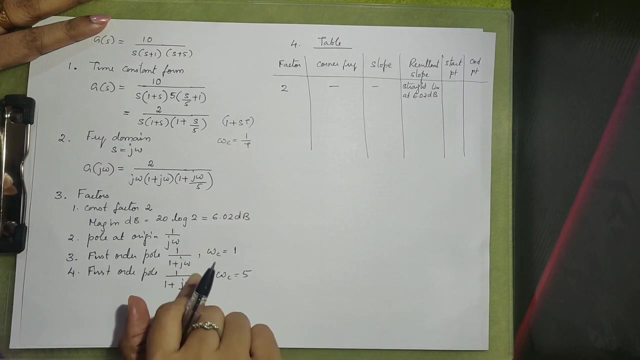 this one is 5, so you need to take one corner frequency. you can take the start point lesser than corner frequency, so i will just take one decade below the corner frequency range. so if omega c is equal to 1 is our the least corner frequency present in the given transfer function. 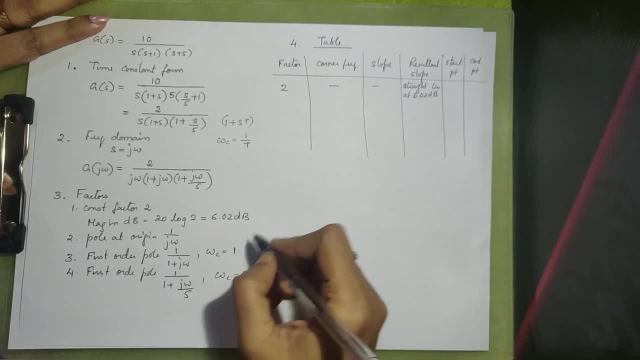 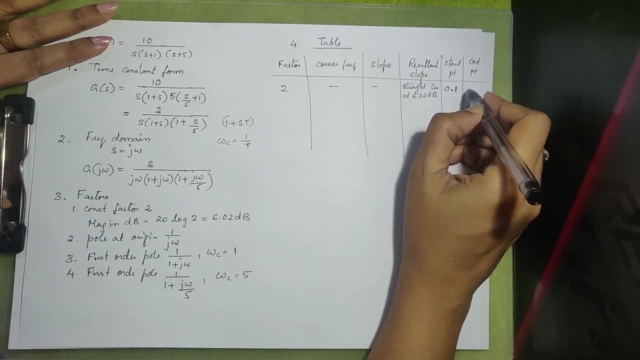 so we will be taking one decade below. so it is instead of 1, we will be writing it as point one. so starting point: we will take it as point one. you can take point zero one also, no issues. so endpoint, actually it will. it will be ending at infinity. the straight line will be going. 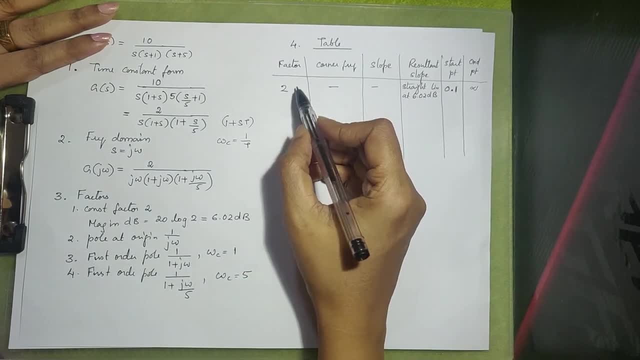 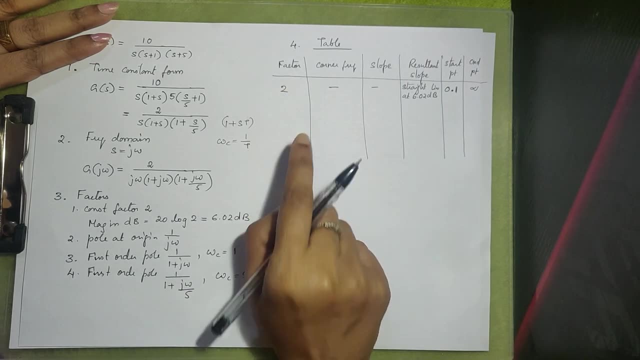 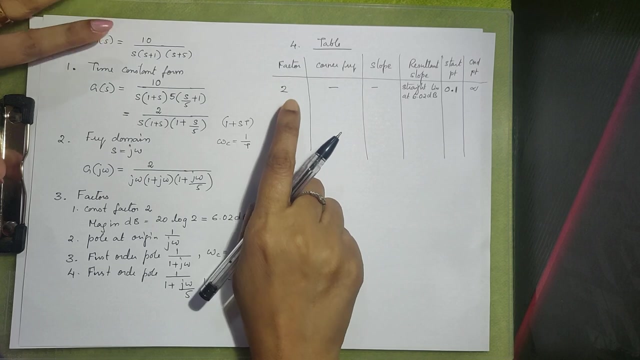 throughout all the frequencies. now when you are writing the factor, you should write the factor in the order increasing order of frequent corner frequency. so when the next factor, if there is a zero or pole present in the transfer function, that factor should come here. so here in this. 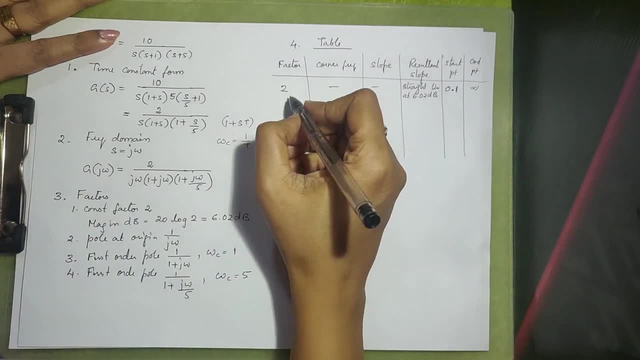 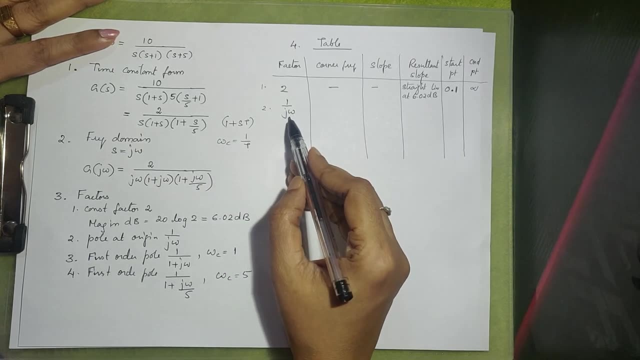 present problem. we have a pole present at the corner frequency. so that is the factor which is 好了 origin. so that corresponds to 1 by j omega. so this is our first factor. this is the second factor, 1 by j omega. so it doesn't have any corner frequency, the slope of this 1 by j omega, as 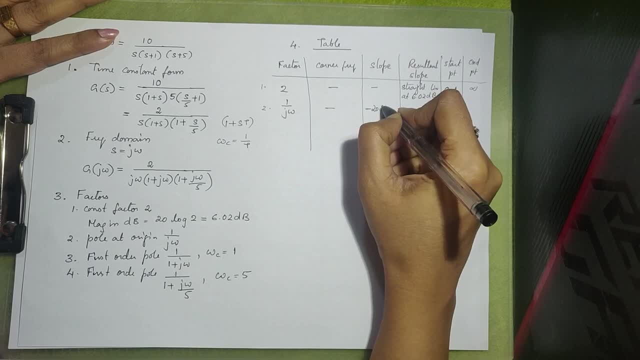 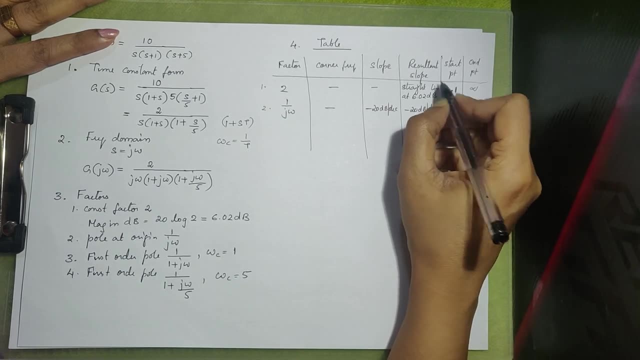 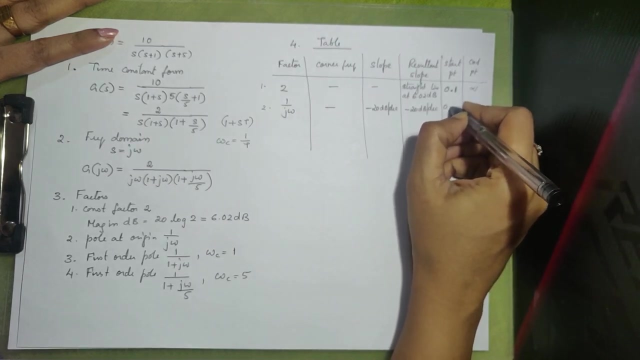 we have seen in the theory it is minus 20 db per decade. so resultant is minus 20 db per decade because there is no other slope present there before this one, because this is a straight line, so the same slope is continuing. a start point is 0.1, then end point. we will keep it blank now. 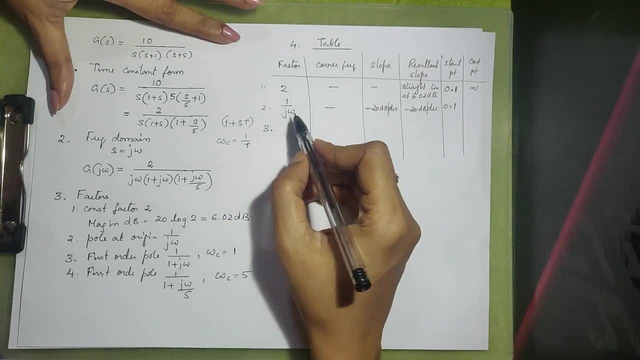 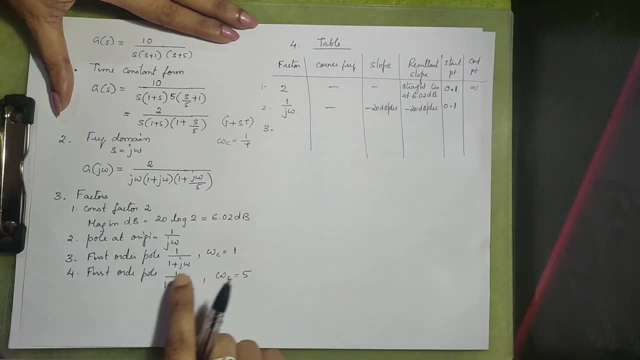 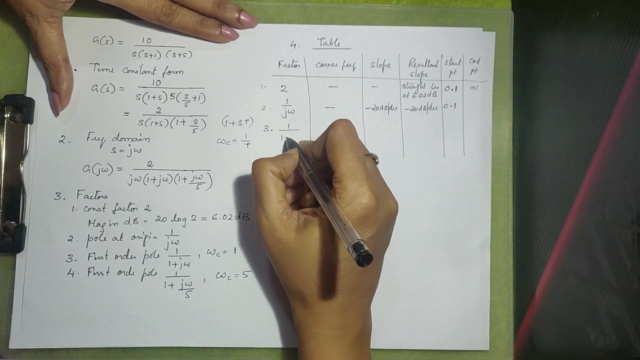 we'll fill the third factor here now. third factor will be the least corner frequency factor should come here. so the least corner frequency factor is the first order pole present at 1 by 1 plus j omega. factor is 1 by 1 plus j omega. what is the corner frequency? corner frequency is 1. 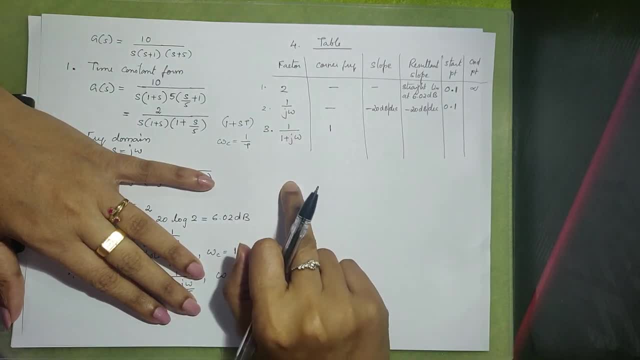 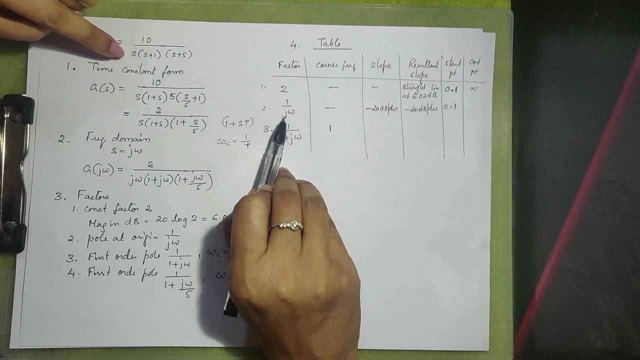 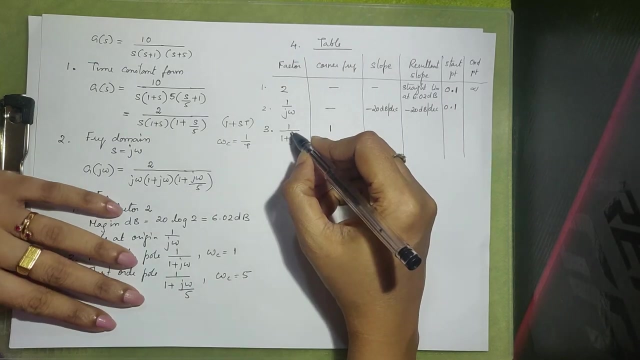 this will be arranging the factors in the increasing order of corner frequency, starting with the constant term pole or zero at origin. in this transfer function pole is present at origin, so that is given. next, then we will be arranging the factors in the increasing order of corner frequency. so for this one, for the first order factor, first order pole, the slope is minus 20. 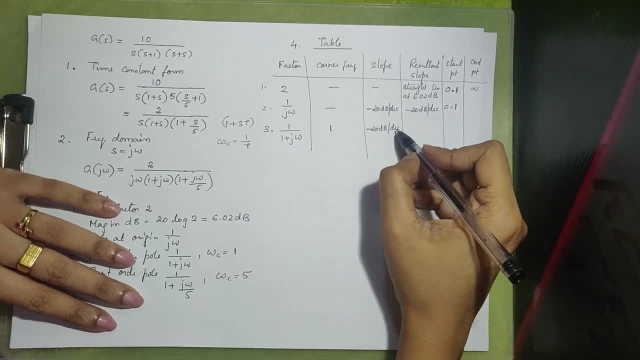 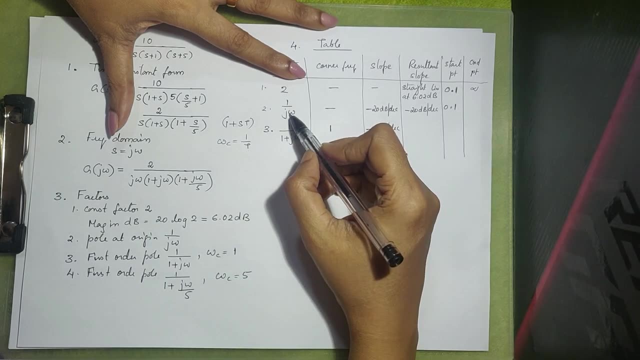 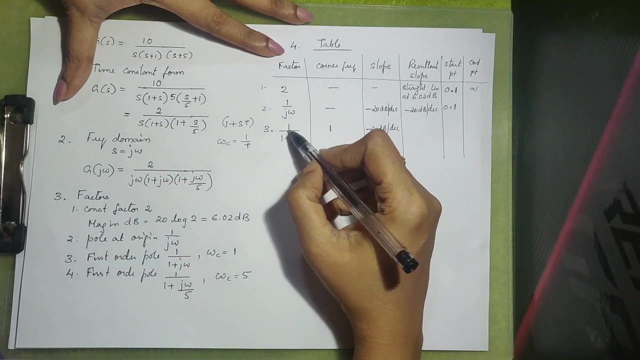 db per decade. that we already know. so now resultant slope here. there will be a resultant slope here. you can see already because of 1 by j omega term, the plot is having a slope minus 20 db per decade. so this slope is for the new term present. so this slope will get added to the 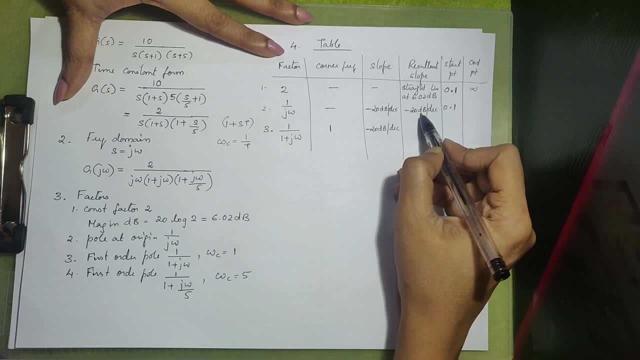 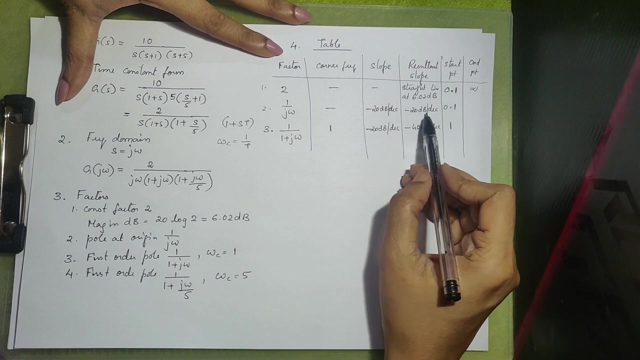 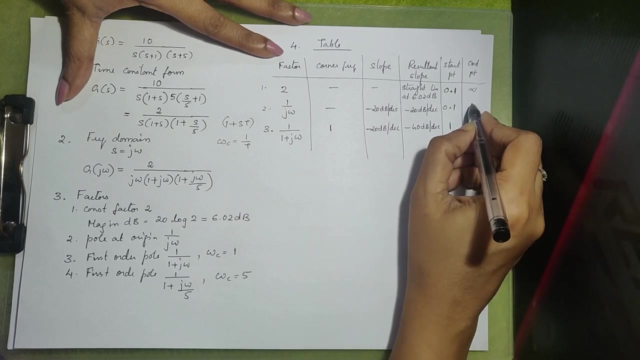 already present slope. so now the resultant slope will be minus 20 db per decade, plus this slope, so it becomes minus 40 db per decade. at what point the slope is changing. at corner frequency 1. okay, corner frequency 1, so here minus 20. the start point is 0.1. at 1 it is changing. means this: this slope is present, only up. 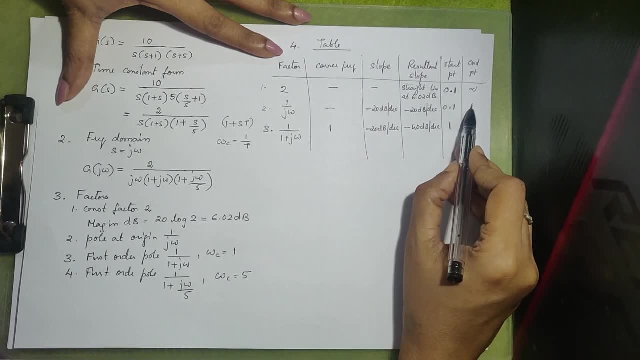 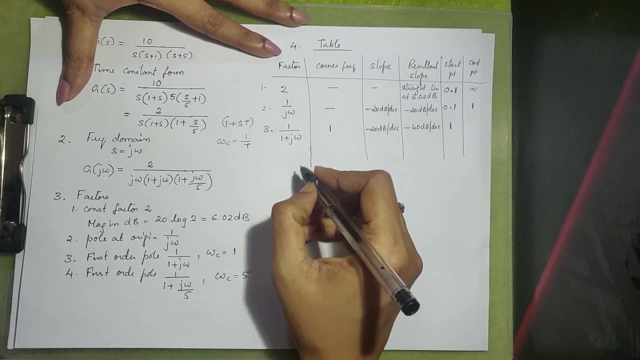 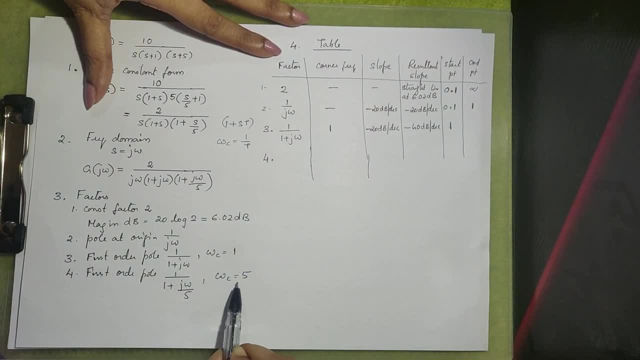 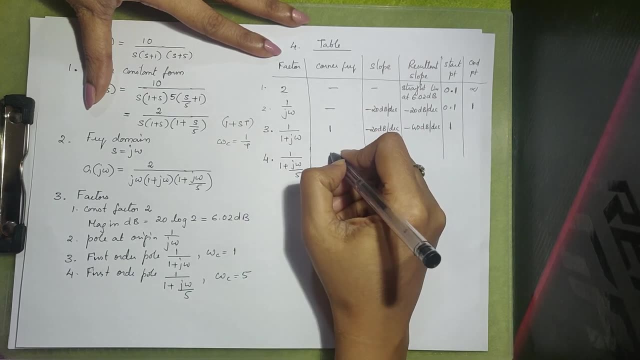 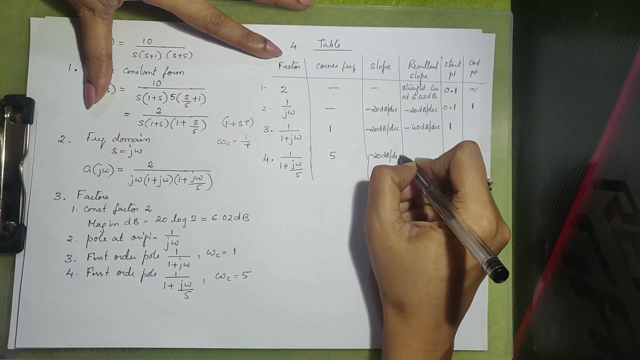 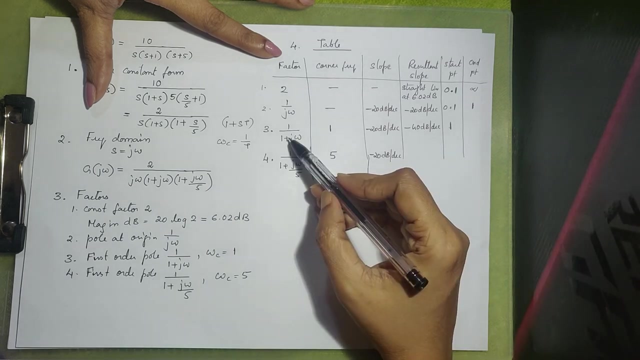 corresponding to corner frequency 5. that is 1 by 1 plus j, omega by 5. what is the corner frequency? it is 5 here. so for this factor also we have the slope minus 20 db per decade. so now already the plot is having a slope minus 40 db per decade, which is due to the term this one and this one. 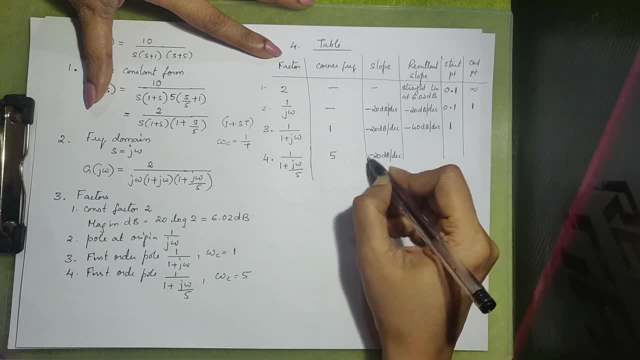 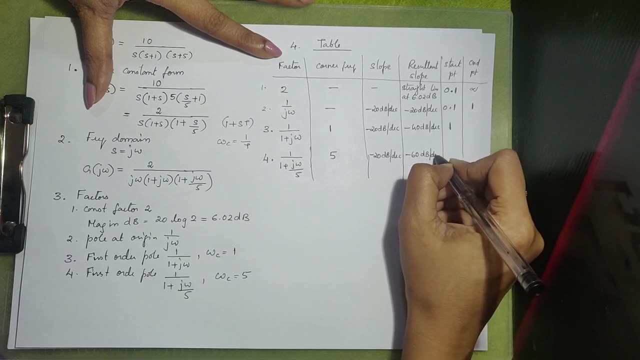 so now this will get added with the current slope. so 40 minus 40 minus 20 will be getting minus minus 60 db per decade as the new slope. now what is the corner frequency corresponding? it is 5. so this, this slope is changing. at what point this? 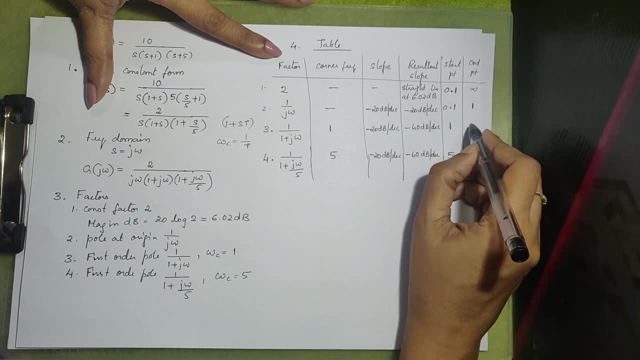 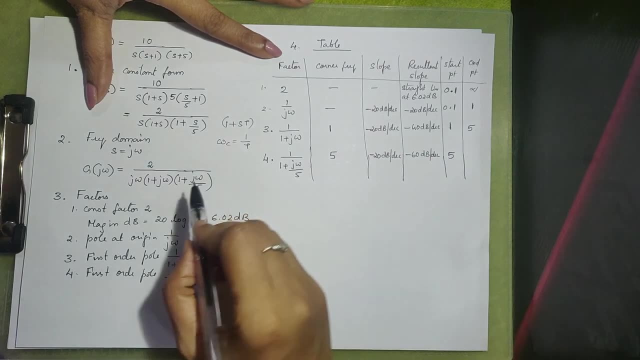 slope is continuing till. we are considering the next factor, so it is next factor. slope is coming at. omega is equal to 5, so this is up to 5, then from 5 it is changing. then we have to check any other terms present. we don't have any more terms present, so we have to check any other terms present. 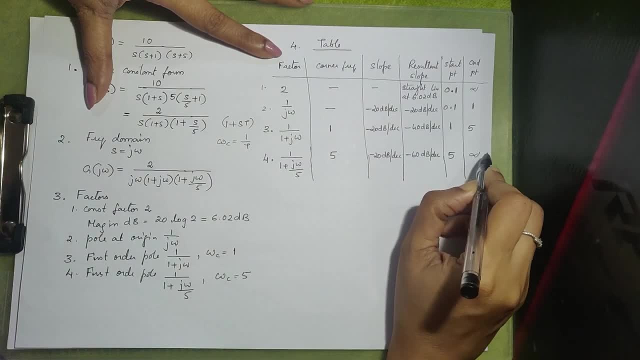 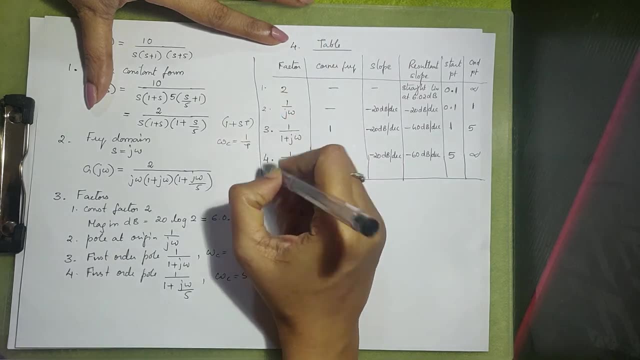 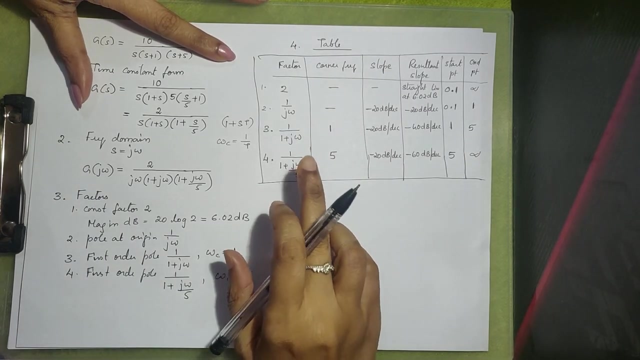 in the transfer function. so this slope will be continuing up to infinity. so our table is ready now. so with this table we will be plotting the bode plot. okay. so now for plotting this. we already know, okay. another thing is: this is for magnitude. so this table is for magnitude now, similarly, we 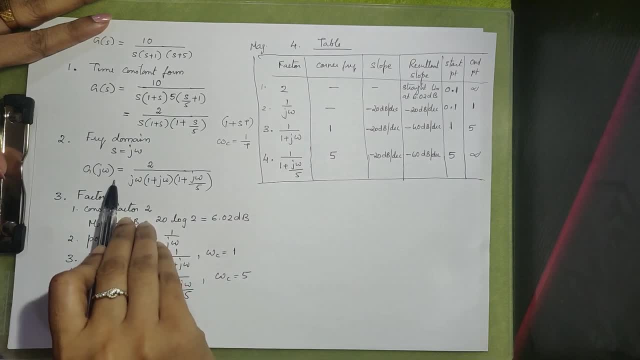 need a table for phase angle. so how will you find phase angle for this one? we have g, j, omega is equal to this one. so this is for magnitude, so this is for magnitude. so this is for magnitude. so this is for. so this is for magnitude, so this is for magnitude, so this is for magnitude. is coming from that passing. 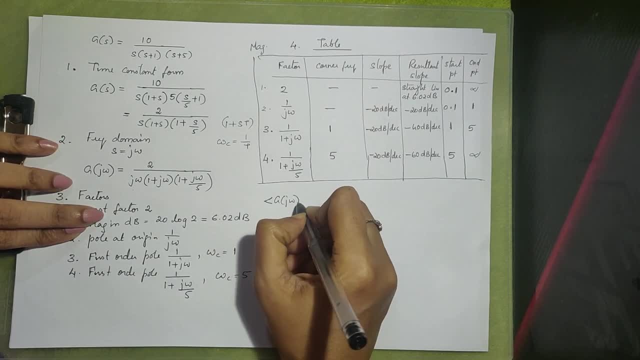 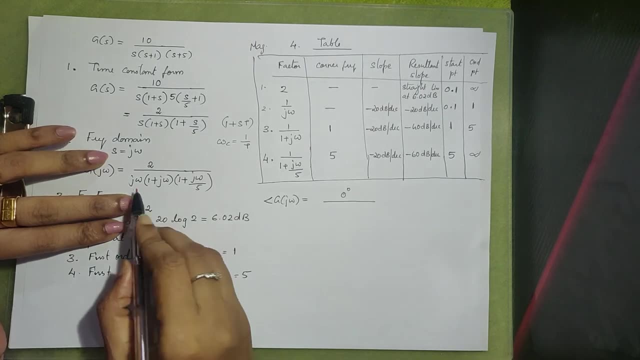 so phase angle angle G j is equal to Who makes aread. so guess what? this is what this U is. so here was also phase angle angle G j. omega is nothing, but in numerator we have zero. degree divided by this is tan Legion 수가 by zero, so will be getting tan. 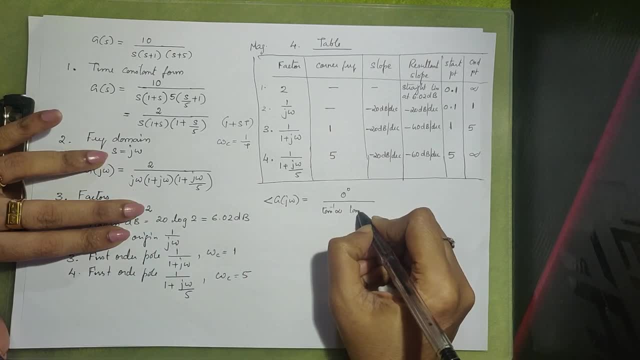 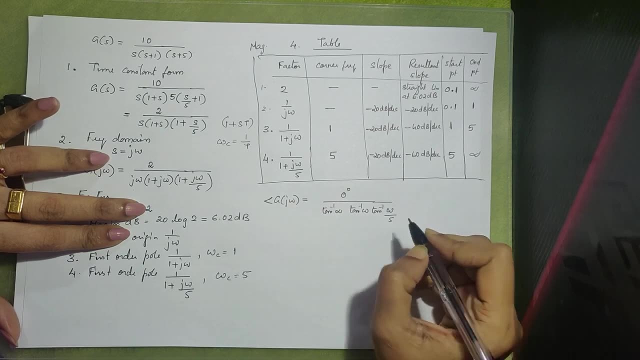 Inverse sup. this is tanwości Tibra, which is negative, and if you reduce this by two, by three times times, we will get this. so this is not negative. and if you do this- otherwise it comes down into this one, this beta- then you will get this a medida. this is a negative in. 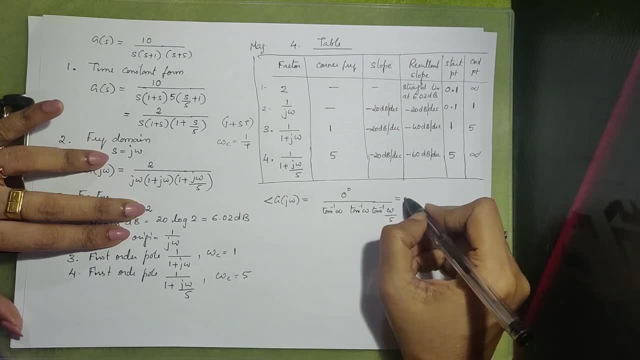 the writing here and this is negative because this is a negative in the children also, and we keep doing so. this aenteprose R基. so again, before we take this to the numerator, we will be getting tan. inverse infinity is 90 degree, So we will be getting it as minus 90. 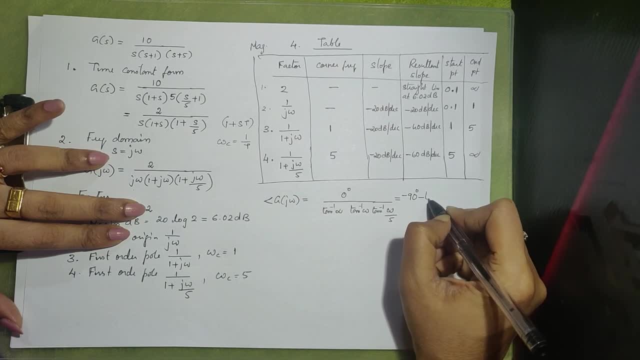 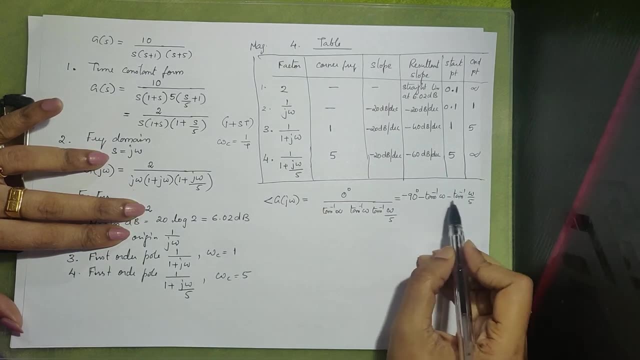 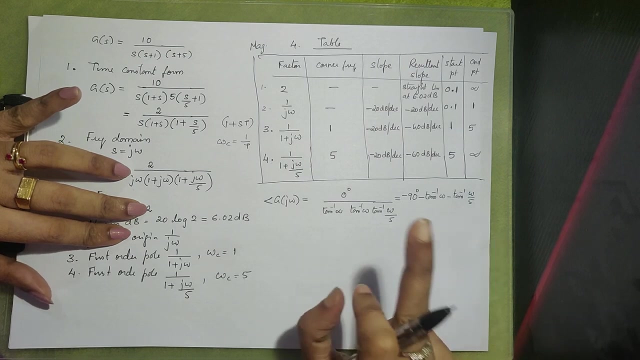 degree to operate in numerator minus tan inverse omega minus tan inverse omega by 5.. So you got the phase angle expression for finding the phase angle: because for Bode plot we will be having two plot, one as magnitude versus frequency, the second one as phase angle versus frequency. 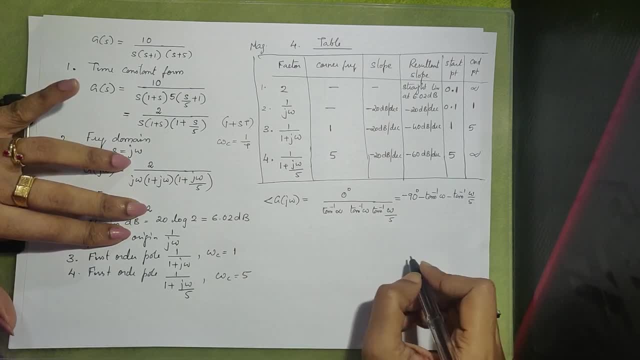 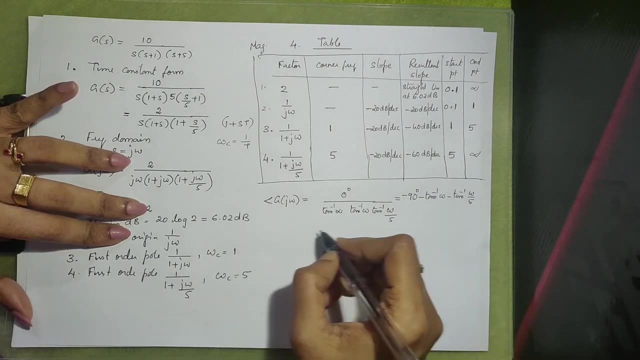 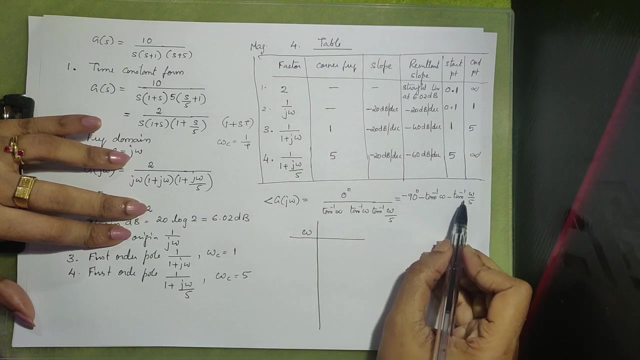 So in x axis we have, we will be taking frequency, which is in logarithmic scale, and y axis will be taking magnitude and phase angle, which is linear scale. Now for plotting phase angle plot, we will be taking omega. what we do, we will be finding phase angle phi for various values of omega. let 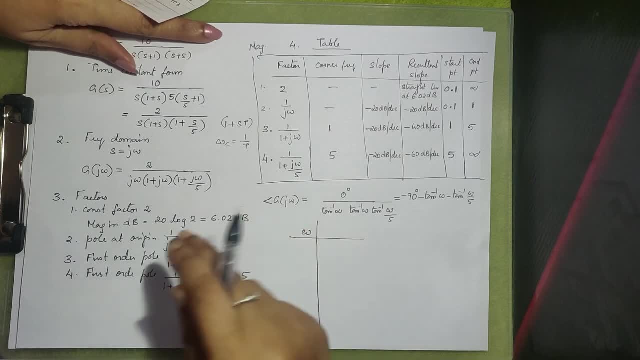 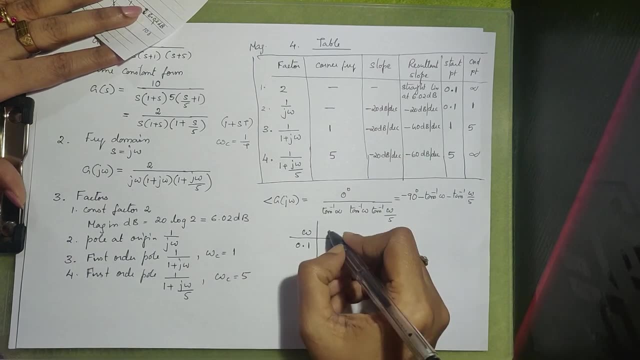 us. it depends. you can start from 0.1, because we have taken from 0.1. So 0.1 here, start point, we have taken as 0.1. So this one, let it be phi- we will be getting when you substitute: omega is equal to 0.1 in this. 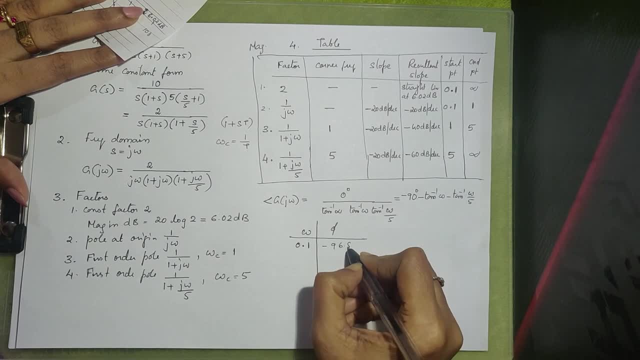 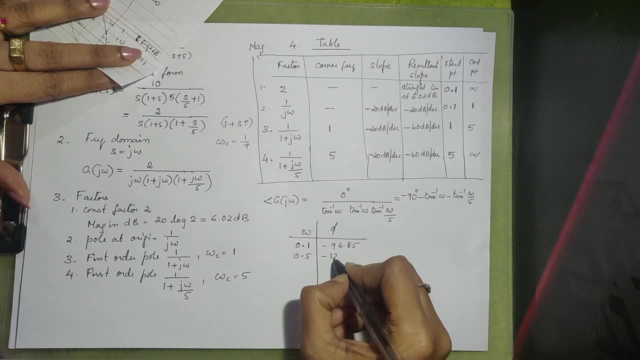 expression you will be getting, and less minus 96.85, then you can increase the value of omega. So for 0.5 we will be getting it as minus 121.66. for 1 we will be getting minus 146.3. for 10 we will be. 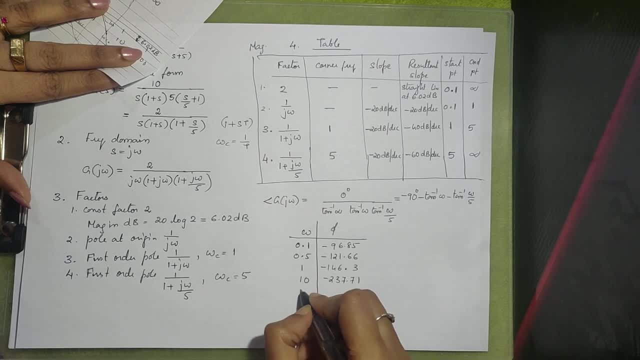 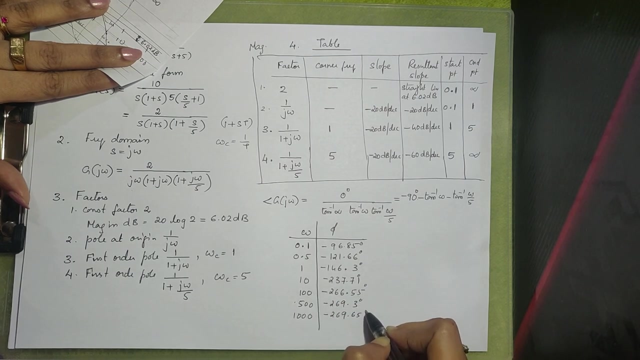 getting minus 237.6.. Take it as 0.81, once again 0.72.less, here 0.70.. Finally, 0.mit 0.MEgW. So you see this lower case here I will be taking to 0.1, and here 1 minus 4 plus 4 is square. 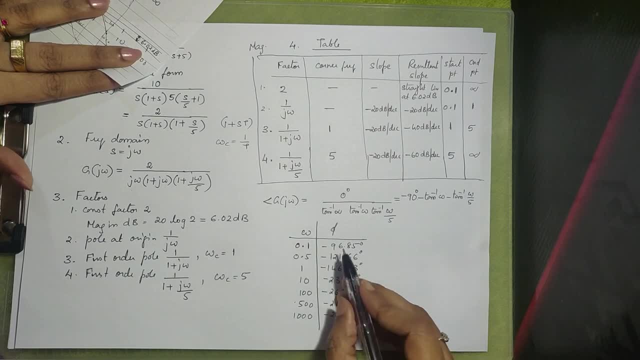 1 plus 4 minus 4 equals to, or minus 4 plus 4.. So, finally, and again, we will take that energía. 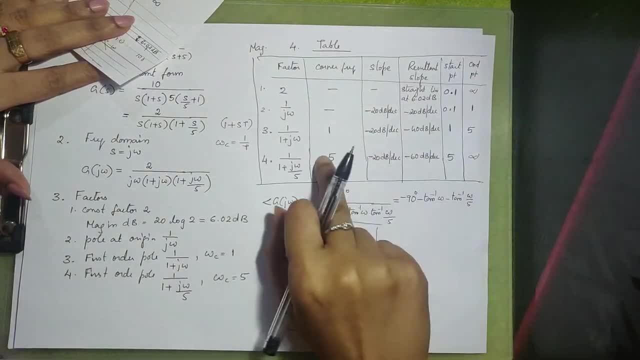 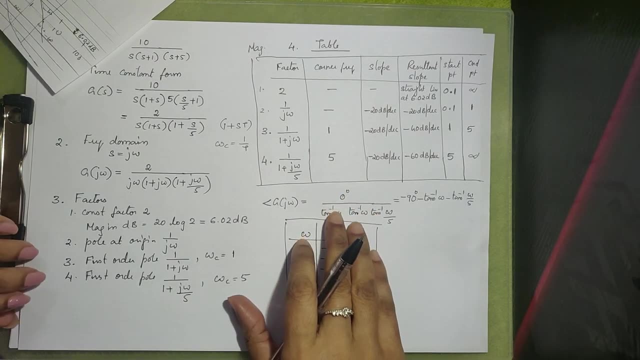 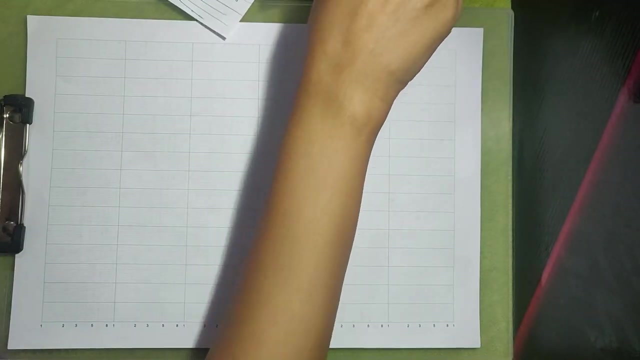 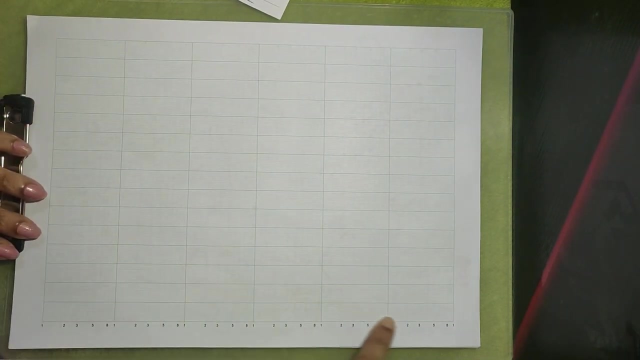 angle. so what we do is now we need: we have the table for magnitude, we have the table for face angle. this one we will be plotting in semi log sheet. so i will take a semi log sheet. this is the semi log sheet. this y axis is linear, x axis is logarithmic. so it is actually. 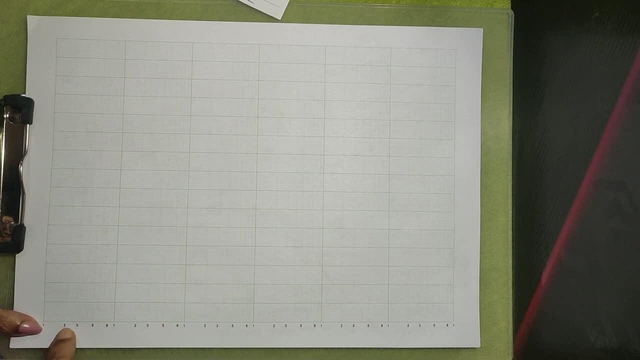 it is not very clear, but here you can see it is marked 1, 2, 3, 5, 6, 1. so this, this much. this is a decade 1 to 1, so it will be starting from 0.1 to 1. so this is a decade, the same value just getting. 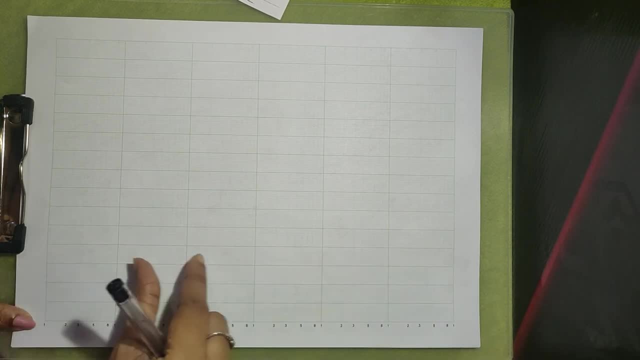 repeated here this much. okay, so this frequency, this value is getting repeated. now, see 1. suppose initial value is 0.1, this will be 1, so it will be in multiples of 10. this is a decade. so 0.1, 1, 10, 100, like that. it goes on. so i can just mark, here we are taking, okay, what we'll do. 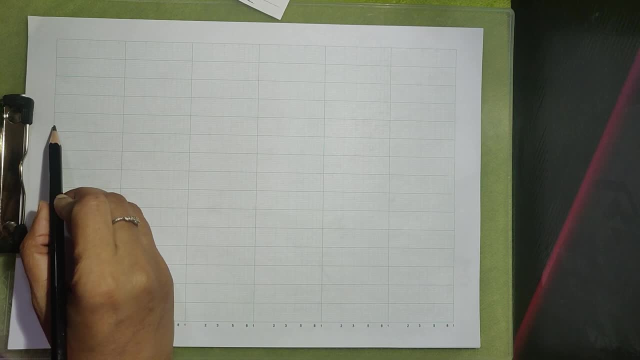 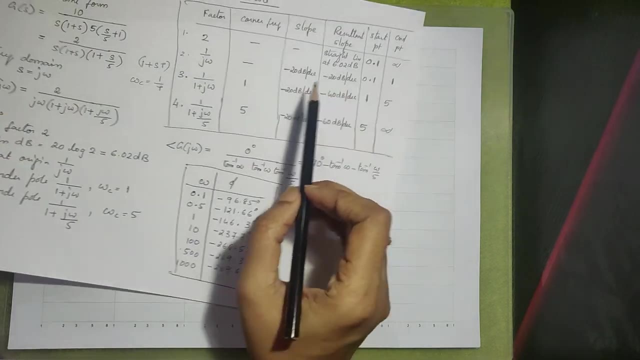 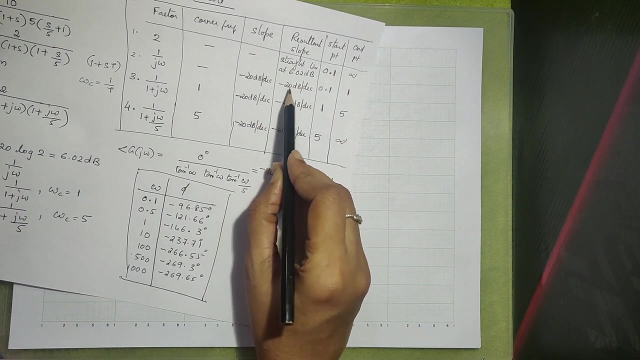 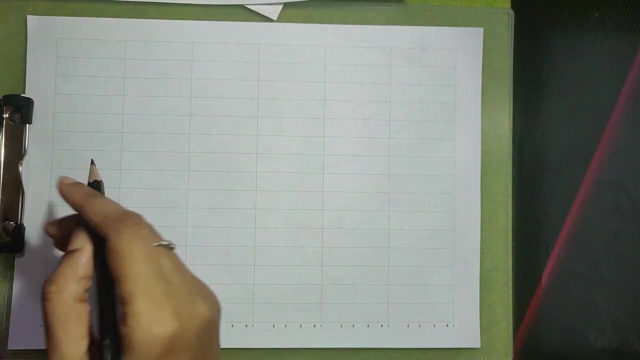 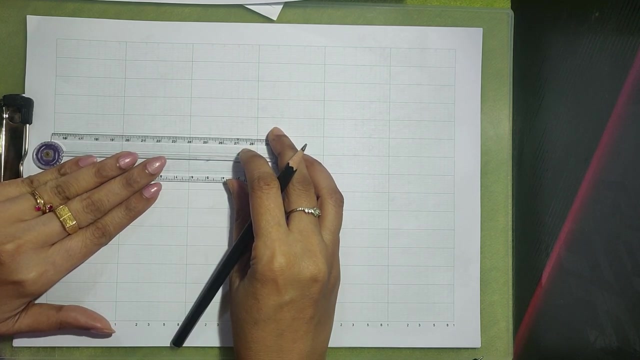 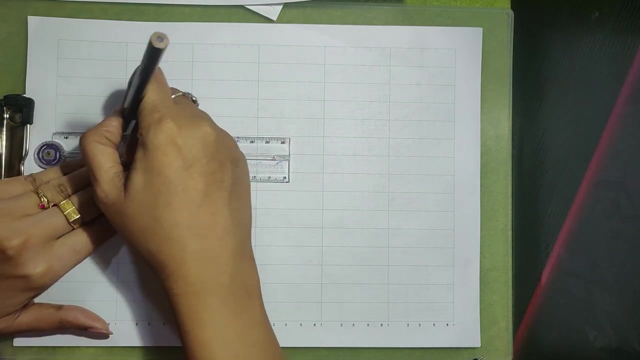 is. i'll just draw a horizontal line: 4 to 60. we need. you just see the table here we need um the slope minus 20, minus 40, minus 60. so we have to mark this as magnitude: 20, 40, 60. So minus 20, minus 40, minus 60. So we need to have enumerator No Top portion. So here we will be. First we need a horizontal line which represents 0 dB. So I am just drawing it, Just draw it. 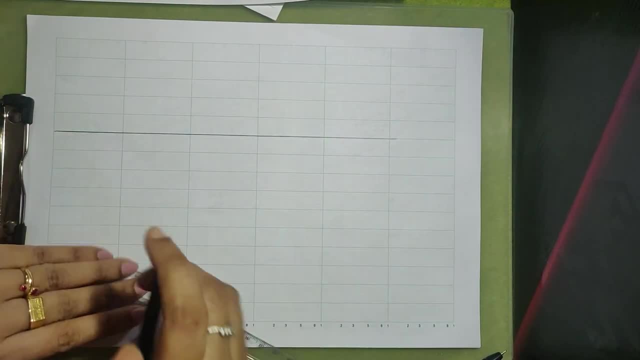 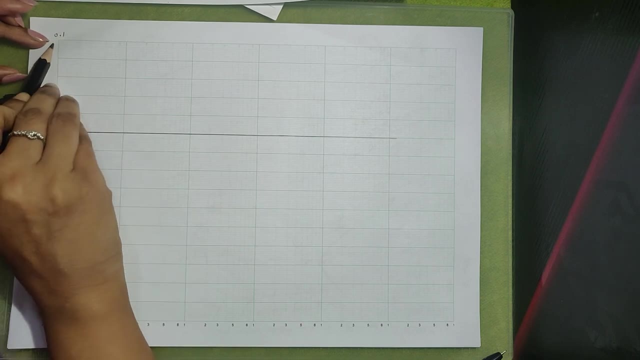 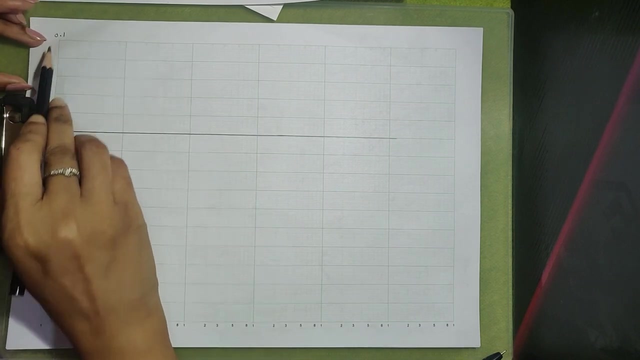 Fine, You don't require that much. So this is actually 0 dB line And we have taken the first point as 0.1.. Starting frequency: we have taken This one. we are marking for magnitude, So don't get confused with this. This is frequency marking, This is magnitude marking. 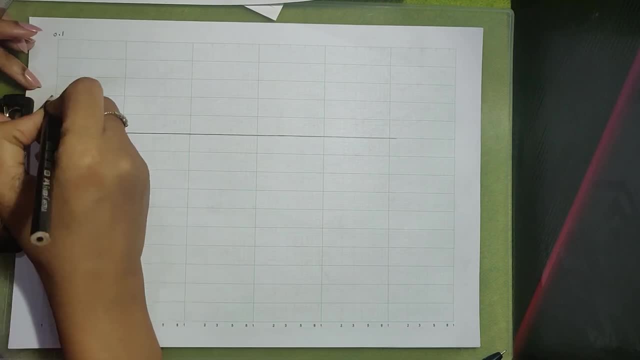 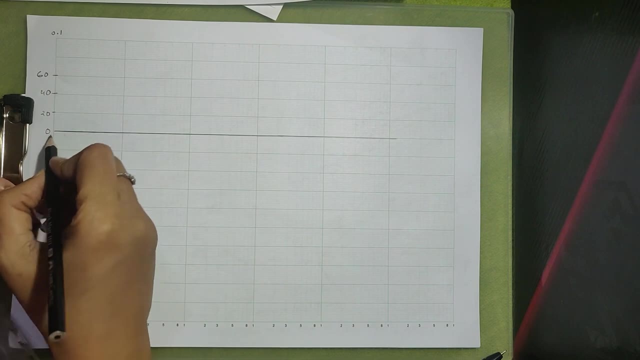 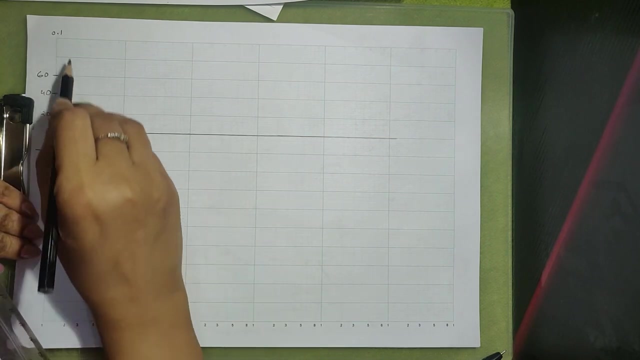 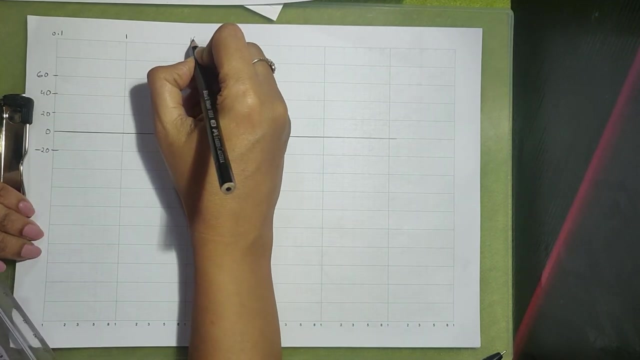 So the next one: here I will be marking 20.. Here I will be marking 40.. Here I will be marking 60.. So in steps of 20 you need to mark. So below this it will be minus 20, minus 40. So on, But we don't require all, So I am just marking. So 0.1 is the starting point for frequency. So second one value will be 1. here This will be 10.. This will be 100.. Like that, This will be 1000. 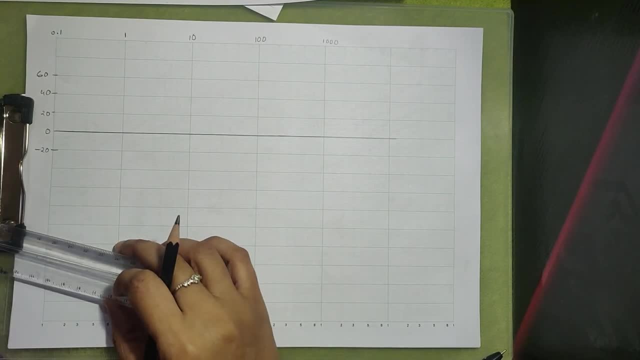 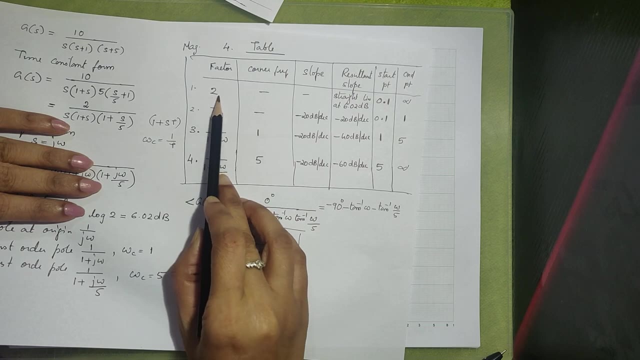 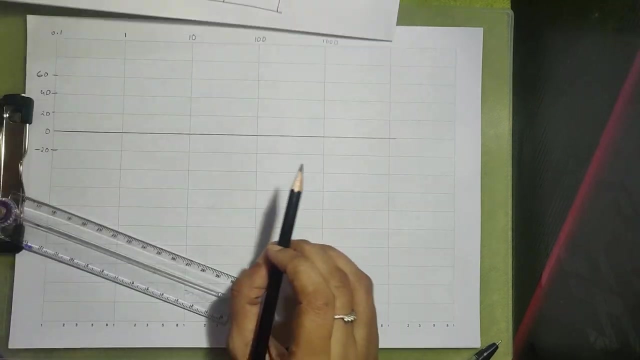 Now what we have to do is we should start from the constant factor here. So this one factor 2.. Constant factor first. 1 is 2. It is a straight line at 6.02 dB. Okay, So we have to draw the straight line first. 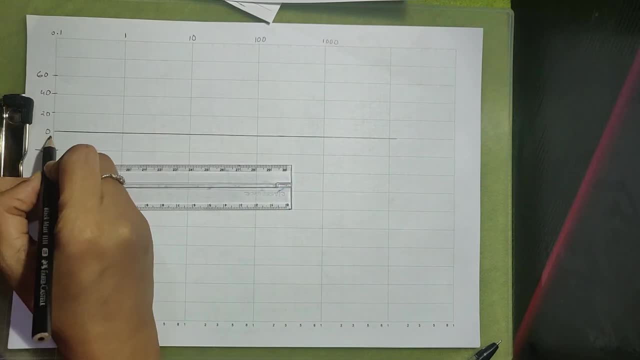 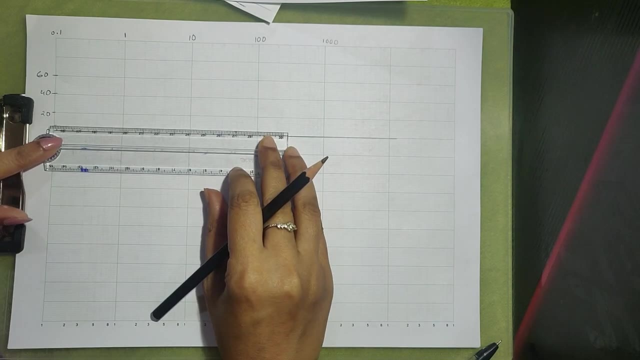 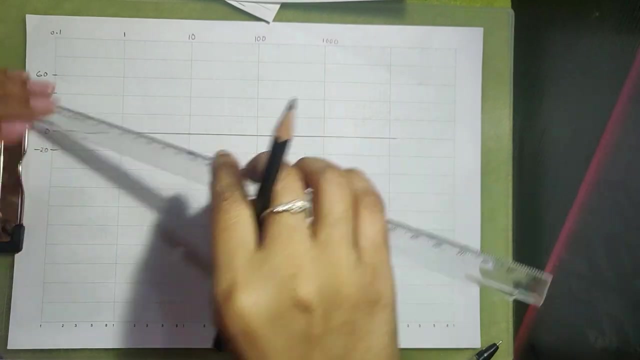 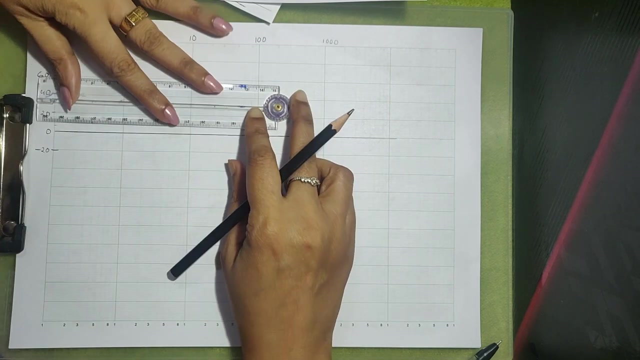 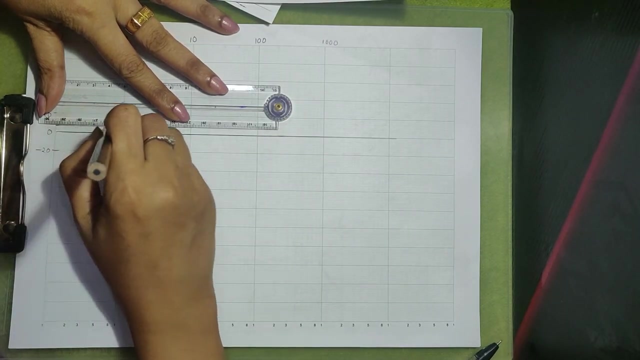 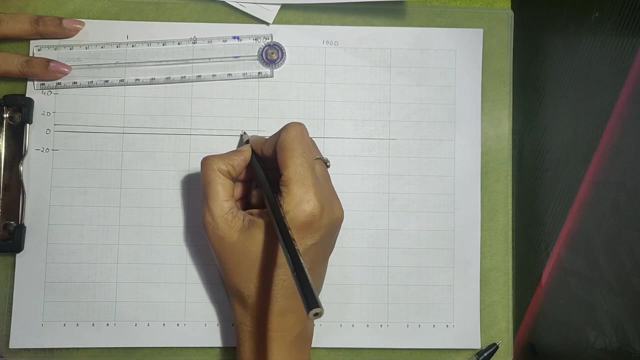 So 6 will be 1, 2.. This is 10.. So somewhere here it will be Okay. I will just mark this. This is the 6 dB line, So this one. This is nothing, but it is 6.02 dB. 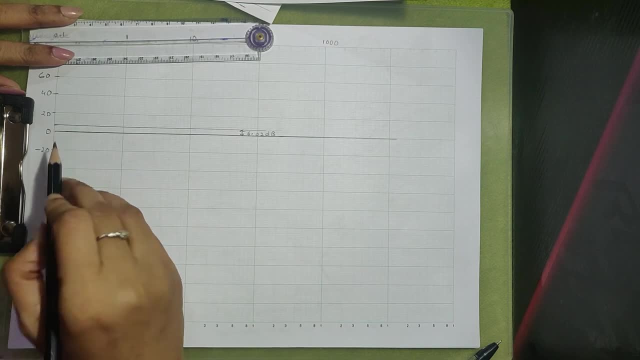 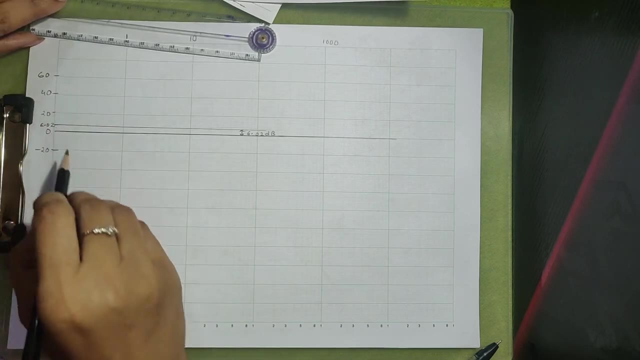 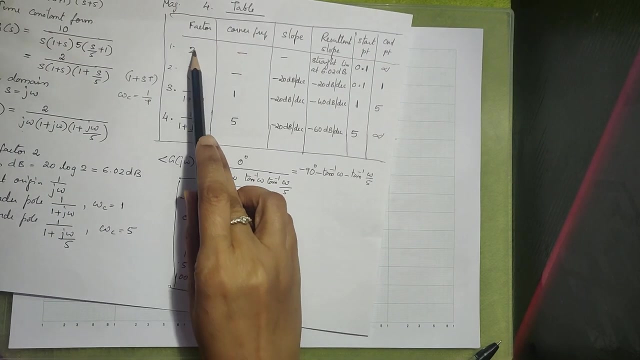 This is the straight line I have drawn at 6.. This is 6.02.. dv this one. so here this is the magnitude, the frequencies. now what we have to do is now see here. so whenever we have the factors here, border plot will always starts with the. 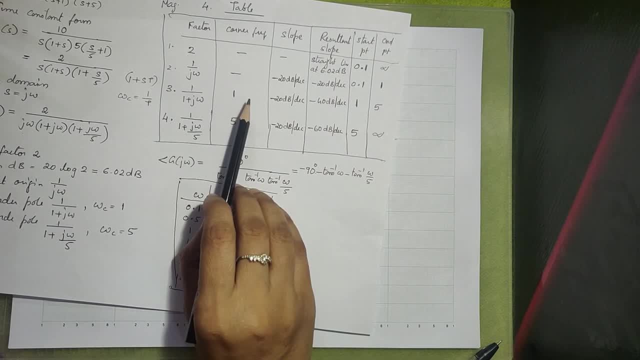 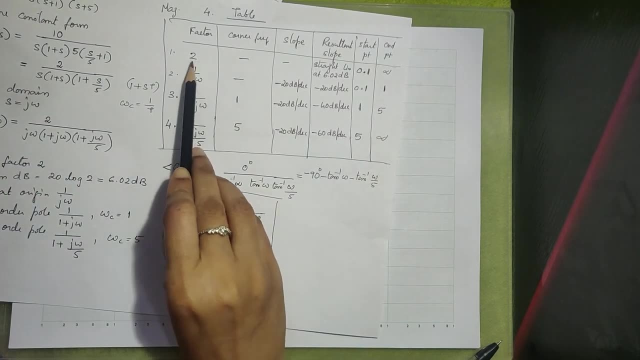 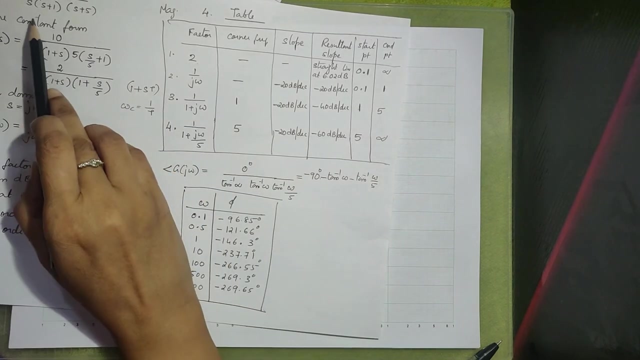 slope which is present for a poles at origin or zeros at origin. so in this particular problem we have a pole at origin that is 1 by j omega. so slope corresponding to that will be the starting slope of the border plot. so starting slope will be based on whether a pole or zero is present at. 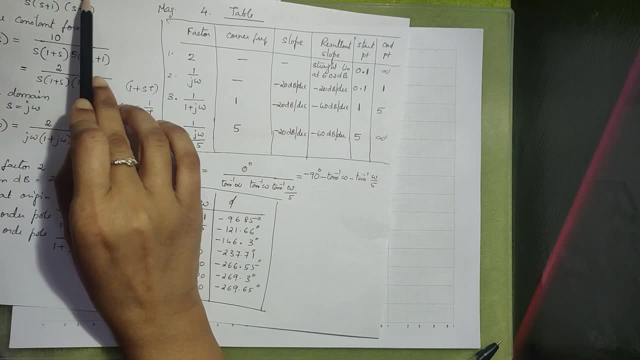 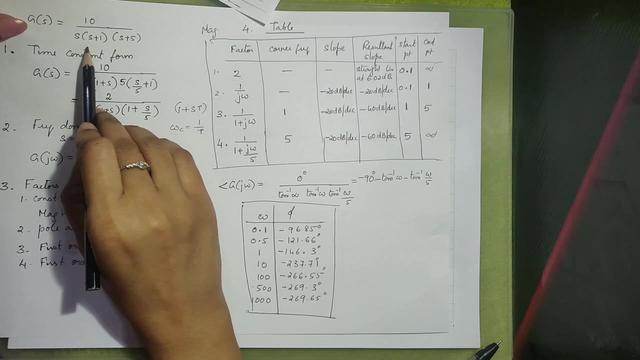 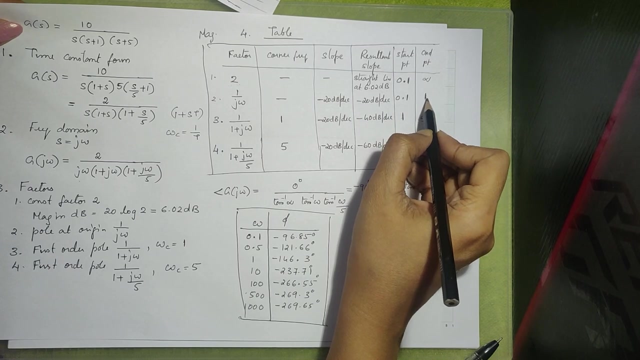 origin. so if zero is present at origin, that means your starting slope will be plus 20 db per decade. here is: pole is present at origin, so the starting slope is minus 20 db per decade. so starting slope is minus 20 db per decade and it is starting from 0.1 and it is going up to 1, ending at 1. 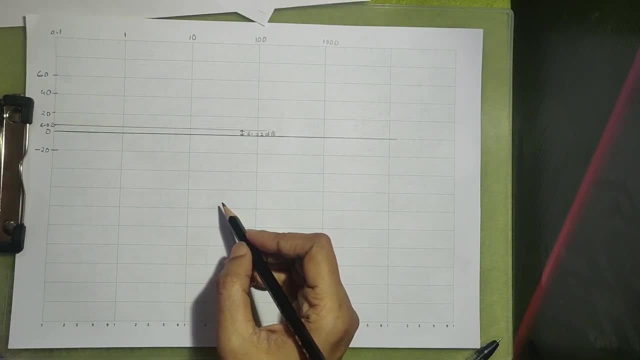 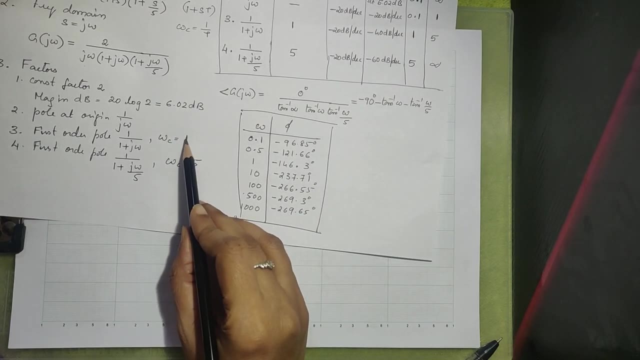 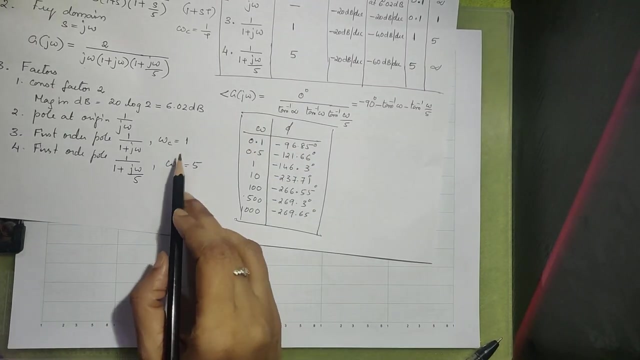 so what we can do is now we have identified the corner frequencies 1 and 5. so just to identify the points where the slope is changing, we will just mark vertical lines at the corner frequency 1 and 5. it is not necessary, but you can draw a very light lines at 1 and 5. so this is the corner frequency corresponding to 1. 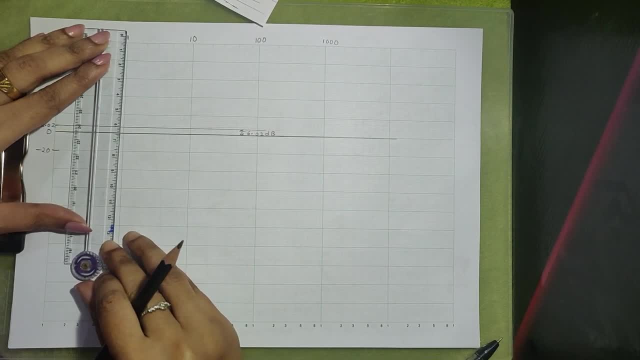 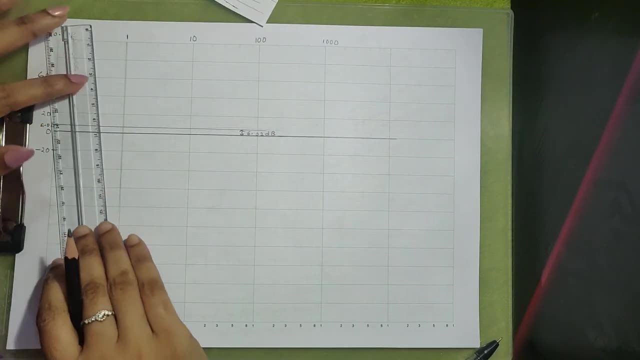 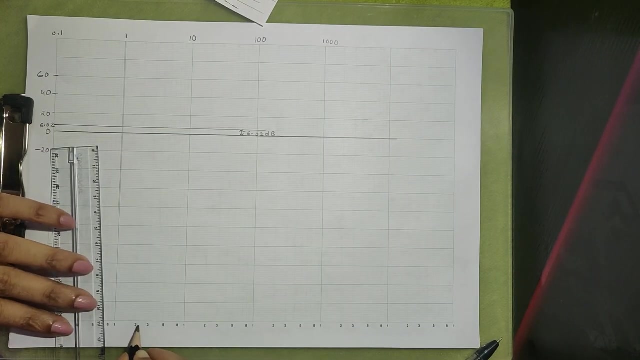 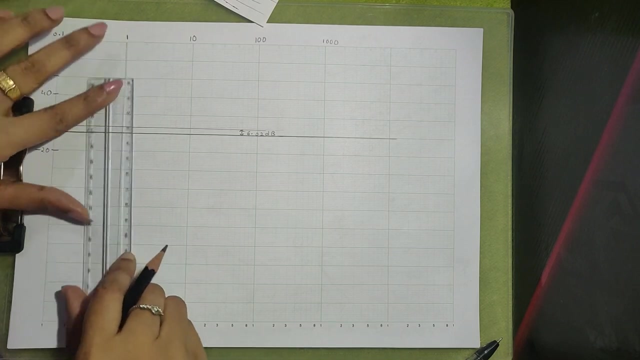 so what i'll do is i'll be just drawing a vertical line there here, very light line, because just for reference purpose, we are drawing that there is a corner frequency at this point. next is corner frequency at 5. you can see, 5 corresponds to here this one. so this line, this corresponding to 5, 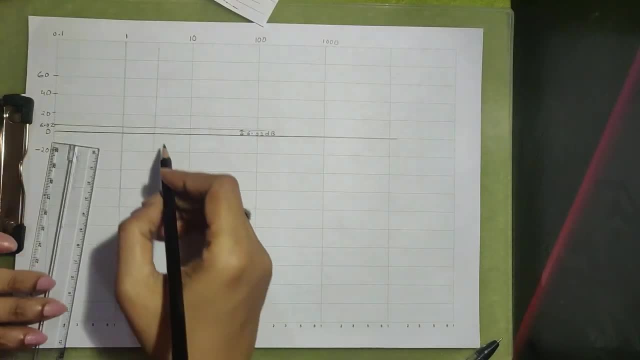 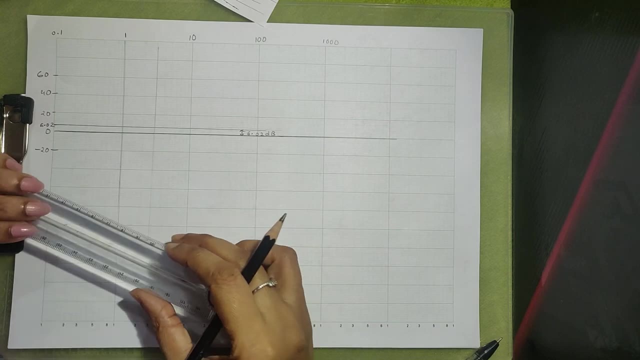 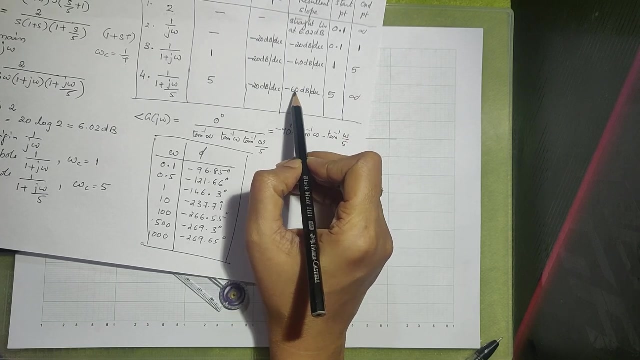 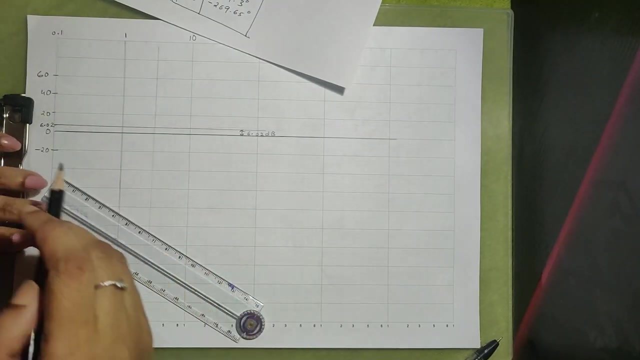 so now you just draw a very light line there. so this corresponds to 5. ok, ok now. starting slope was minus 20. so we have a lines of slope minus 20, minus 40, minus 60. so what we do is we need to have lines of slope minus 20, minus 40, minus 60. so first we will draw those lines. 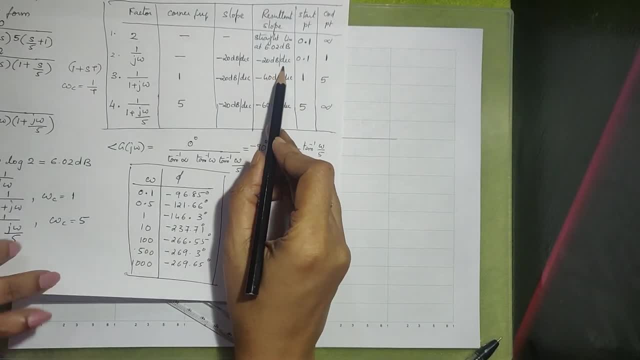 this one is 1, so it is db per minus 20 db per decade. we know this is a decade, so for getting minus 20 db per decade, slope what we do us, this one is added for this line, so this数 is 10 and 20 is 40.. 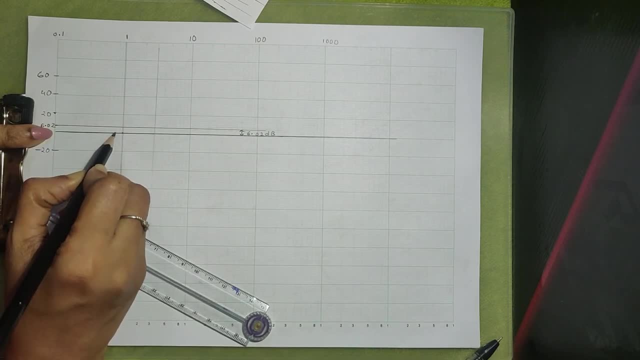 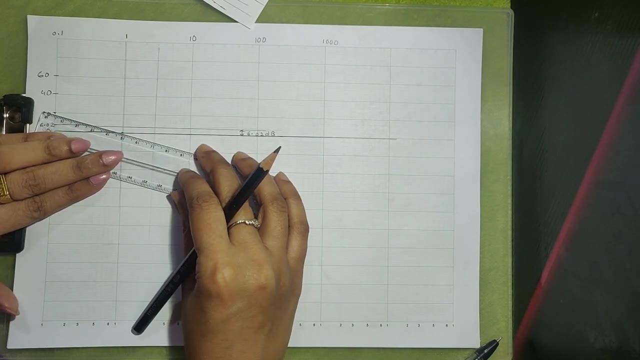 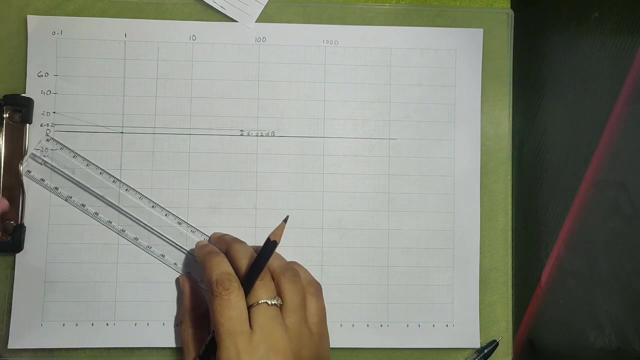 do is: this is 20, this is the horizontal, which is corresponding to a decade. so we will draw a slope here which corresponds to. this is also very light line. please draw very light line because this is for our reference purpose and for getting minus 40 db per decade. what we do is this 40 and 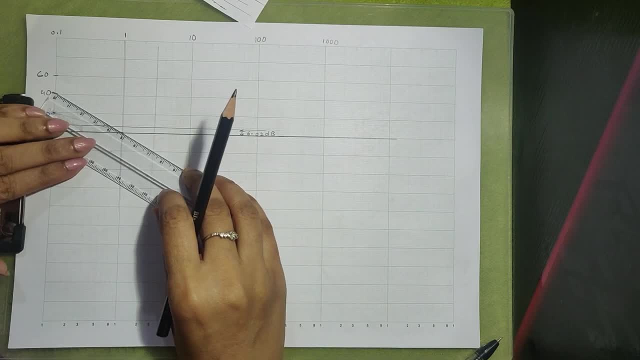 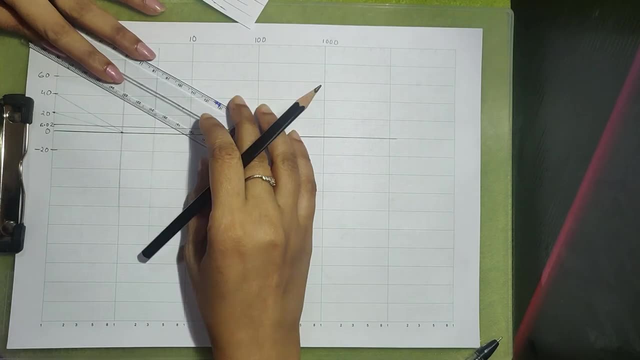 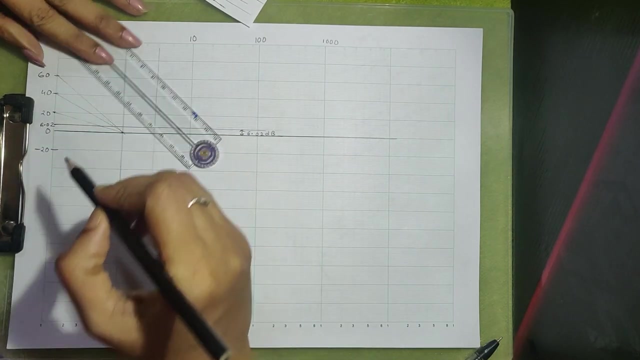 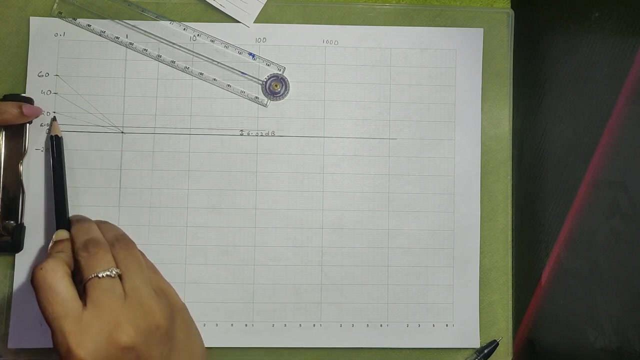 this one we will join. so we are drawing like this. then we have 60 db per decade line. so we got three lines: one, two, three. what i have done this is the decade first decade. so join this 20 and this point horizontal reference point, we will be getting minus 20 db per decade. 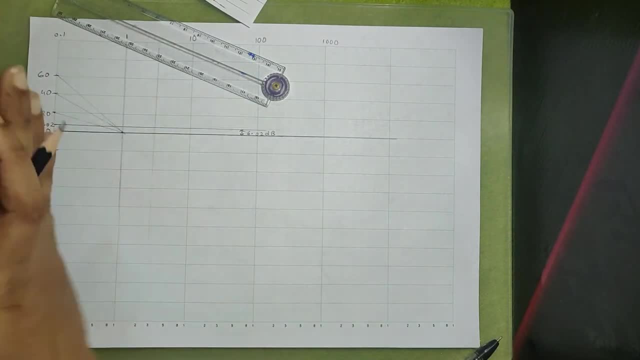 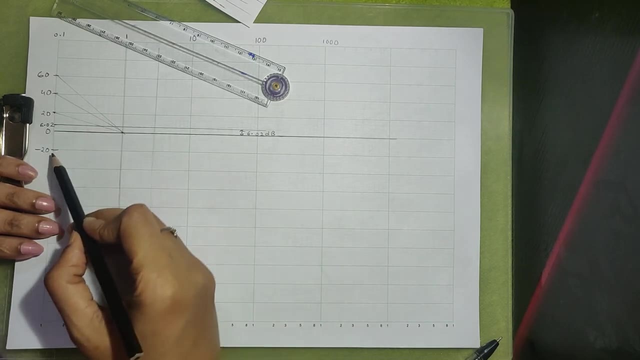 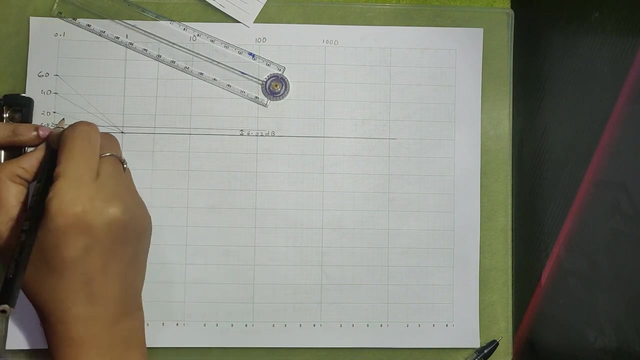 line see. negative slope is always in downward direction. positive slope means it should be in upward direction if it is plus 20 db per decade. you will be drawing like this: this: you will be joining this 20 and this one. so it's a positive slope here it is a negative slope. so now this: 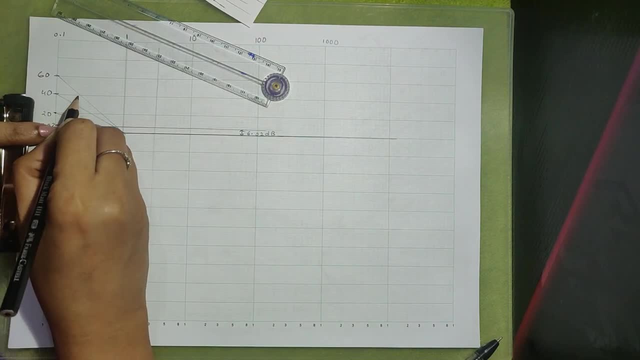 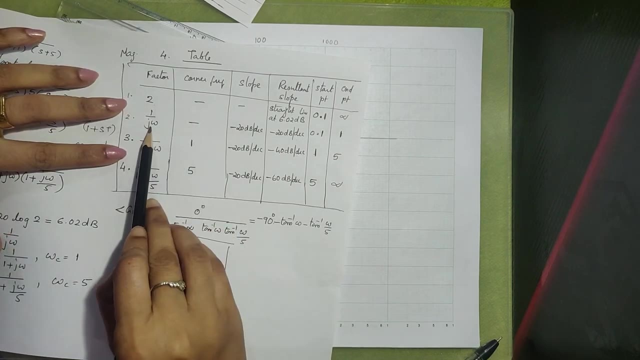 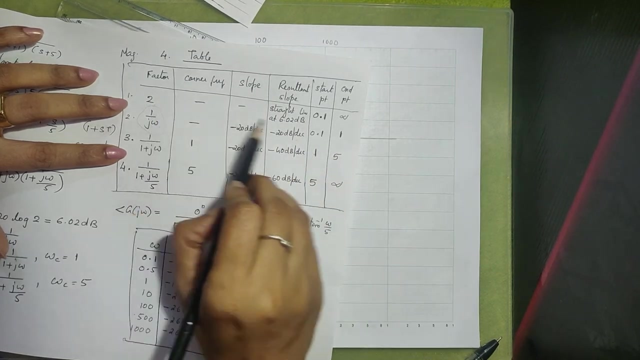 represents minus 20 db per decade. this is minus 40 db per decade. this is minus 60 db per decade. one thing you need to remember is here, this, this point, this, our starting slope, is minus 20 db per decade and it is starting at 0.1, but at the same time, we need to satisfy this condition. also, what? 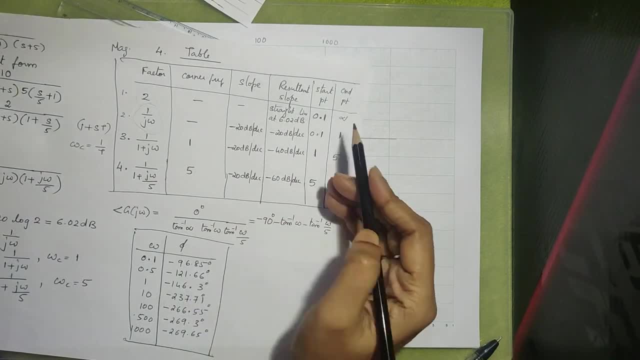 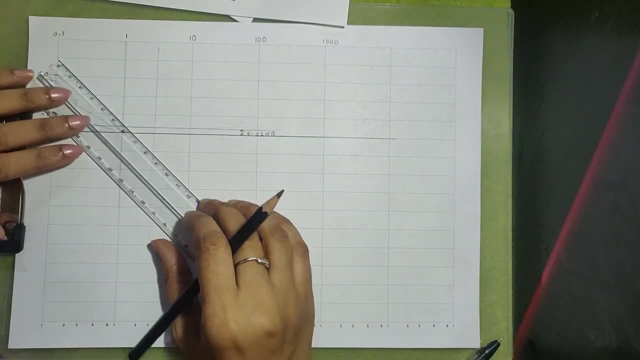 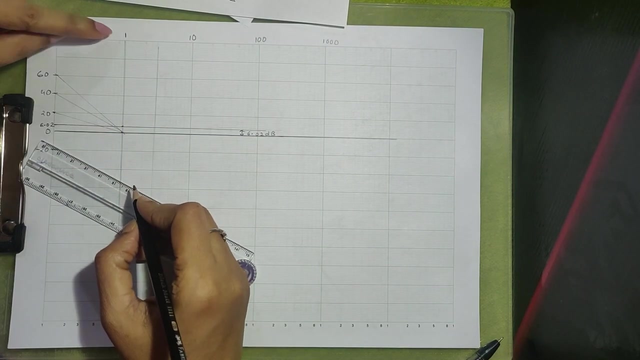 is this condition: magnitude is 6.02 db and here the slope is ending. starting point is 0.1 and ending at 1, so at omega is equal to 1. actually omega is equal to 1, the magnitude should be 6.02. that means the magnitude should be this one. so this is the value corresponding. this is omega. 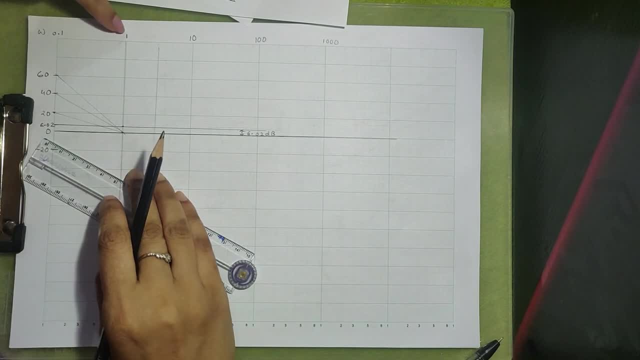 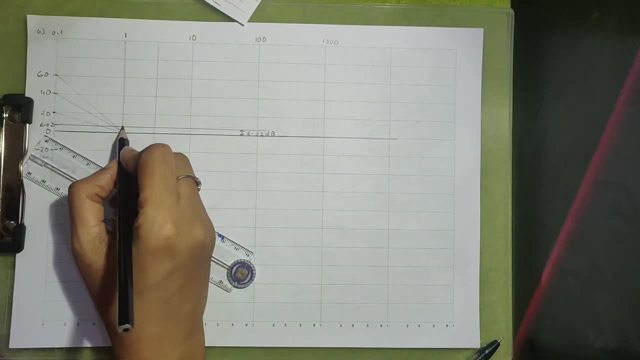 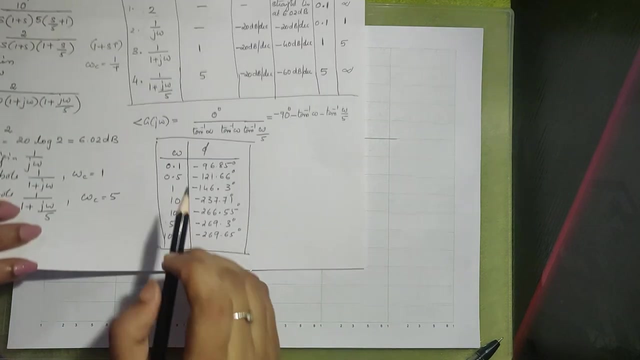 this is omega 0.11, 10. so for omega is equal to 1, our magnitude should be: magnitude is 6.02, so 6.02 should be the magnitude. but at the same time we should have a slope, a line of slope minus 20 db per decade at that point. so this 20 db per decade line, 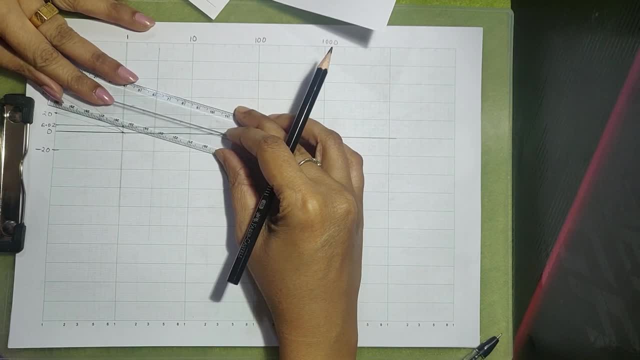 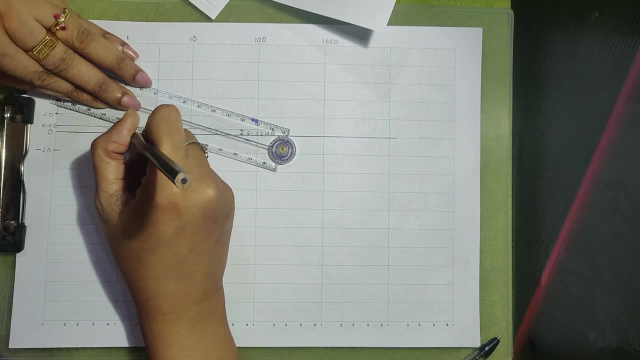 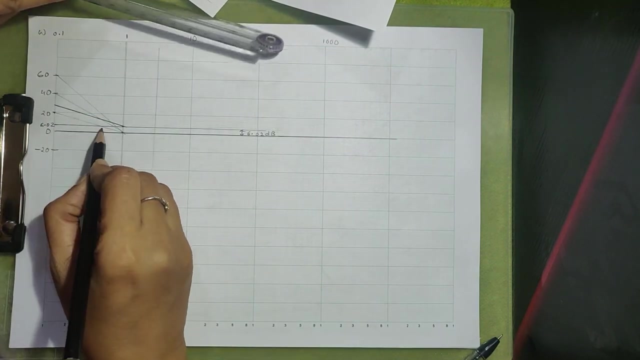 we should have a slope of minus 20 db per decade, and this is the value corresponding to this already have here. what we do is we draw a parallel to that one, a dark line which is up to 1. this is this: this line represents this line minus 20 DB per. 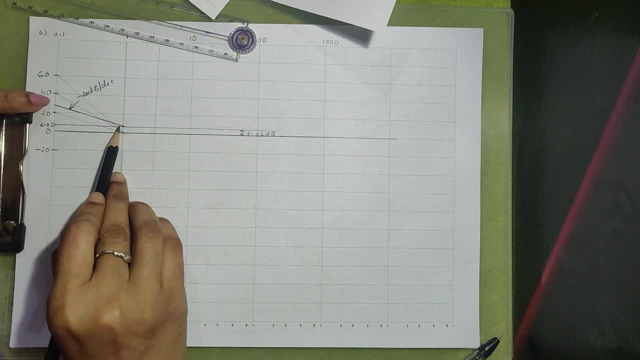 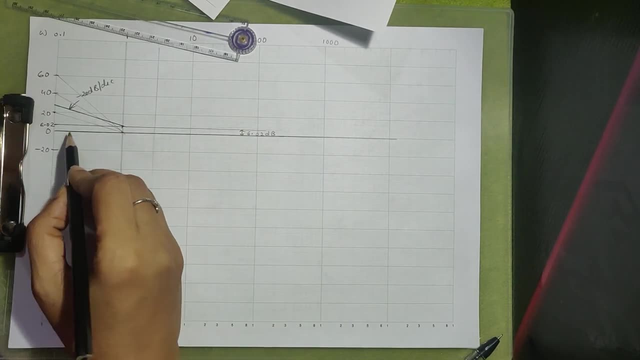 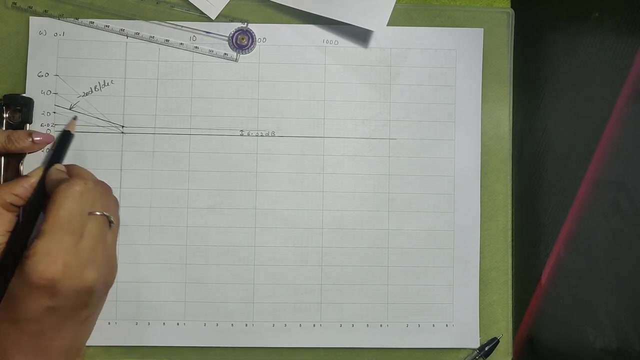 decade. this is a minus 20 DB per decade line passing through 6.02 DB at Omega is equal to 1. so how we draw, we have drawn this line by. we already have a minus 20 DB per decade line here which we have already drawn. the slope draw the. 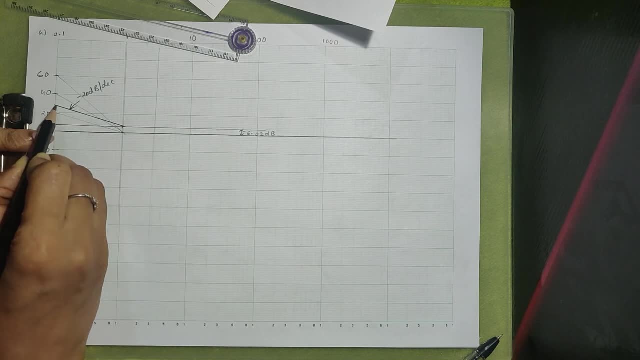 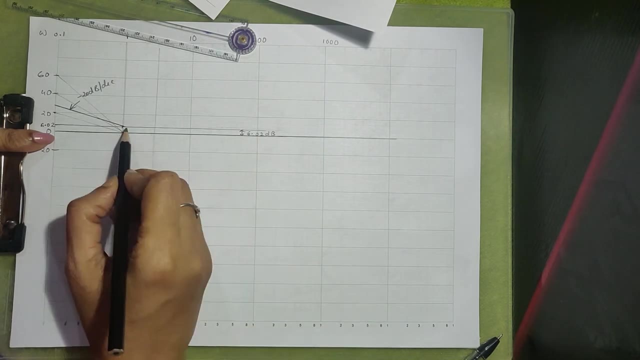 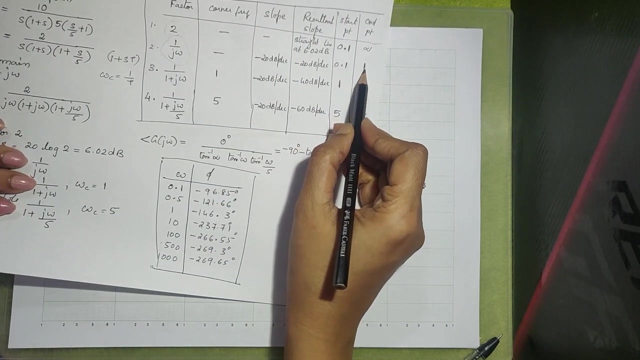 parallel to this minus 20 DB per decade line, so that the parallel line drawn should pass through this line intersectionally. 6.02 at omega is equal to 1 and we already know from this table that slope. this one is 0.1 up to. 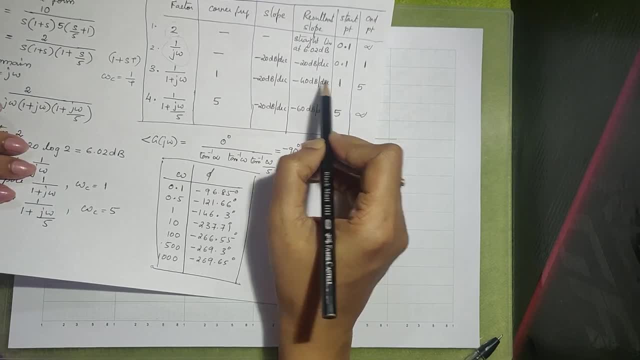 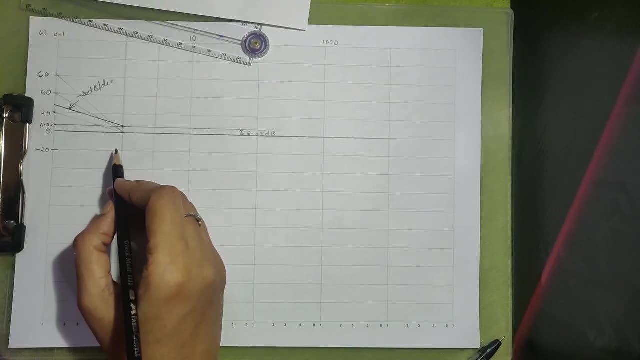 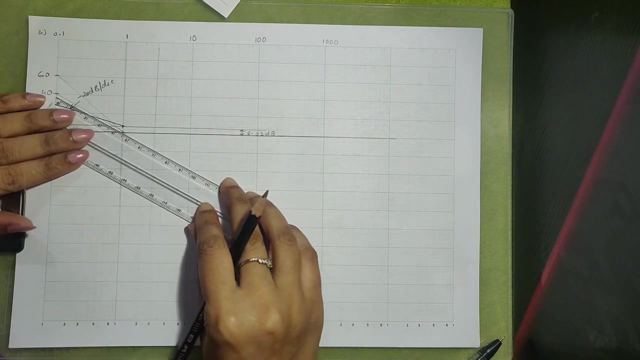 n point is 1. so at 1 corner, frequency 1, what should be the slope? now? minus 40 dB per decade, and it should continue till frequency 5, so this one. at this point now the slope should change to minus 40 dB per decade. so this is our 40 dB per decade line, this one. so what we do, we will be. 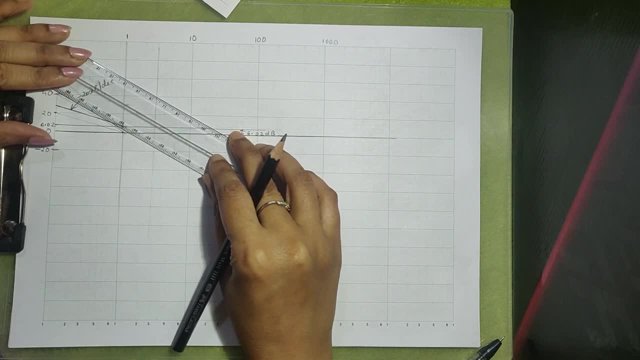 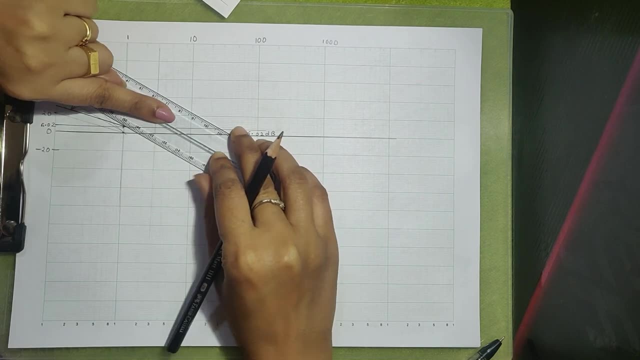 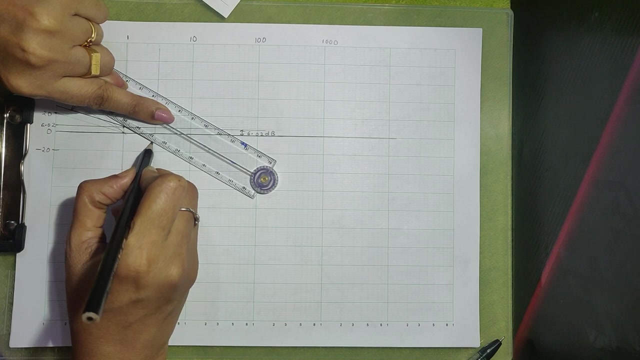 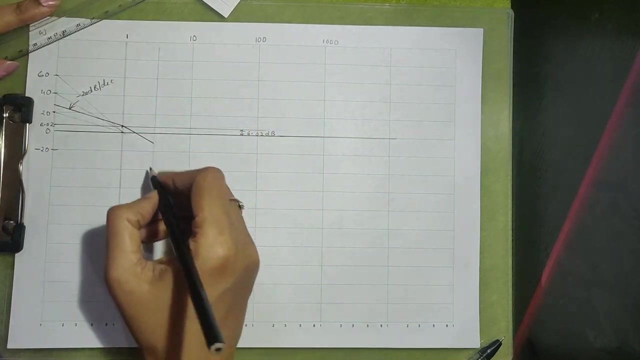 drawing a parallel to that line. this is minus 40 dB per decade. we will draw a parallel to that line and so now we got a 40 dB per decade slope line and it should be minus 40 dB per decade till. the omega is equal to 5, so this is 5 corresponding to 5. so we are stopping here now. now, what will happen at? 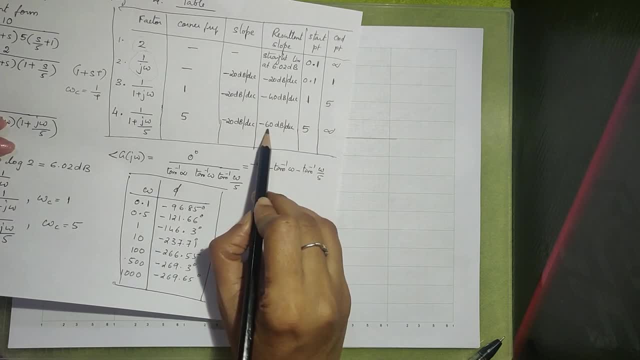 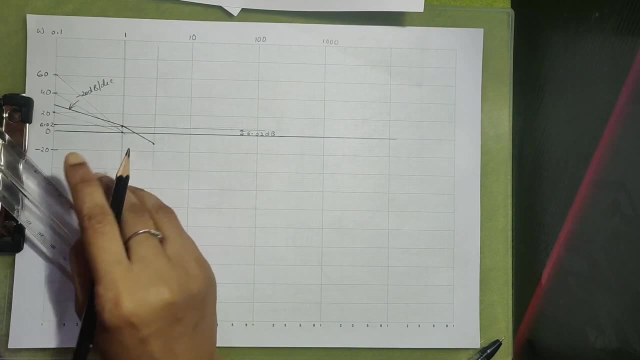 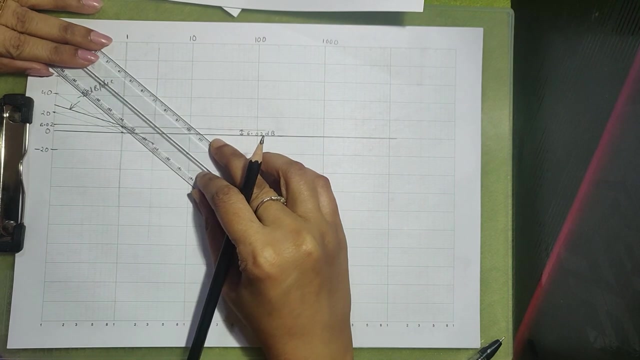 5. at 5, what happens? starting point: the slope is changing to minus 60 dB per decade. now we will be we. at this point we should have a line at 60 dB per decade line. so this is our 60 dB per decade slope. this one is 60 dB per decade. 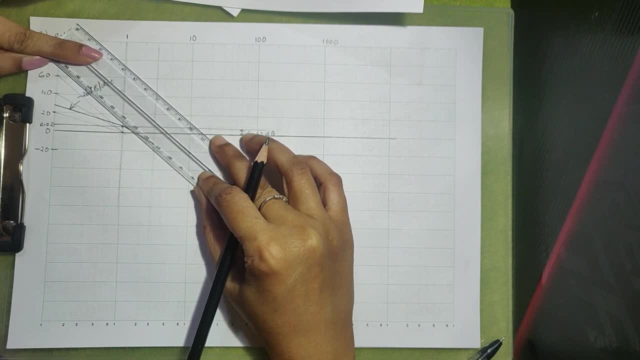 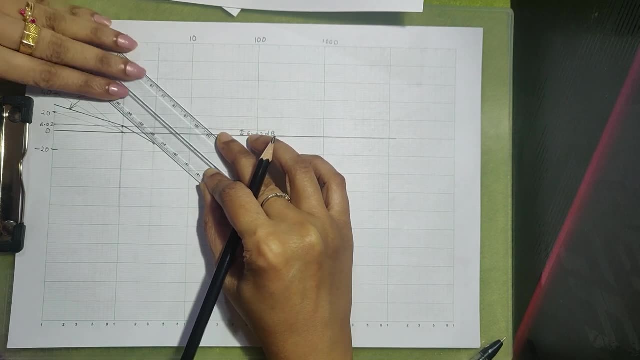 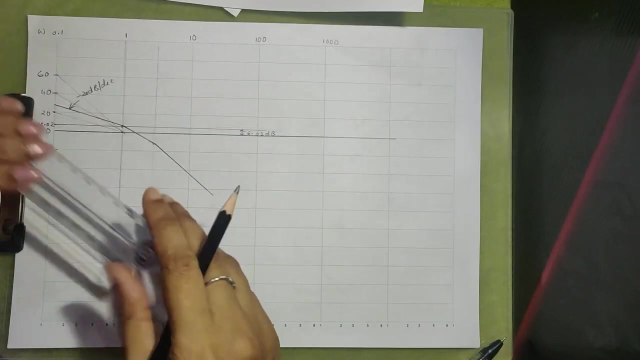 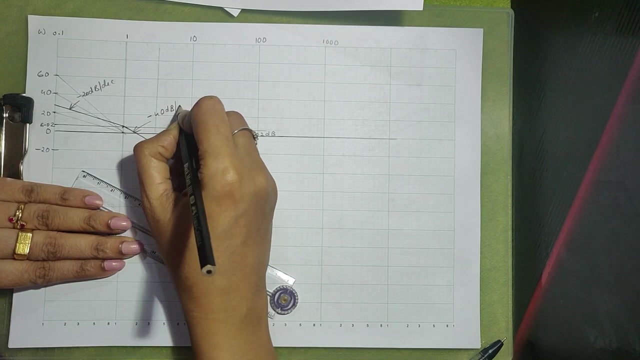 We will cry. yet parallel to 60 dB per decade, starting from Omega is equal to 5. this is just approximate, I'm drawing so we got the value there. So this actually basically now here: this one is minus 40 dB per decade and this one is minus 60 dB per decade. 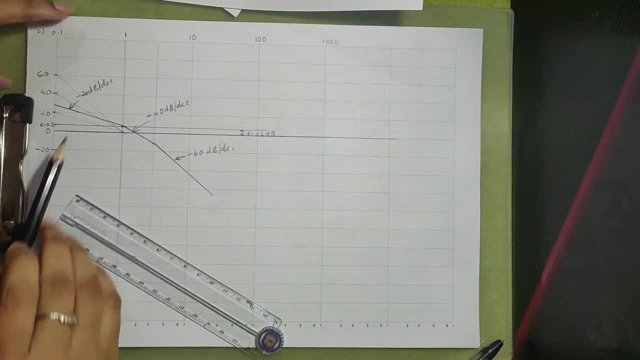 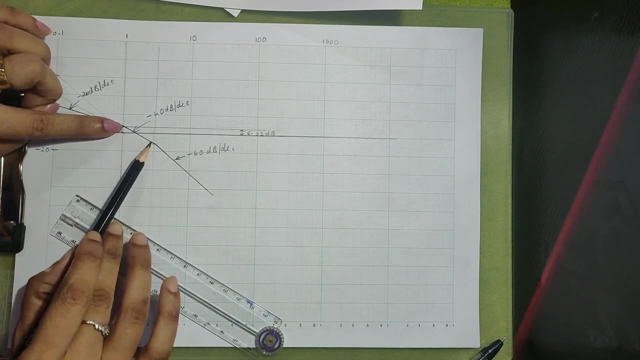 per decade. so we got a magnitude plot. now here the first portion, initial portion, starting with minus 20 db per decade going up to the first corner frequency. at first corner frequency slope is changing to minus 40 db per decade. then it is going to the next corner frequency. there the slope 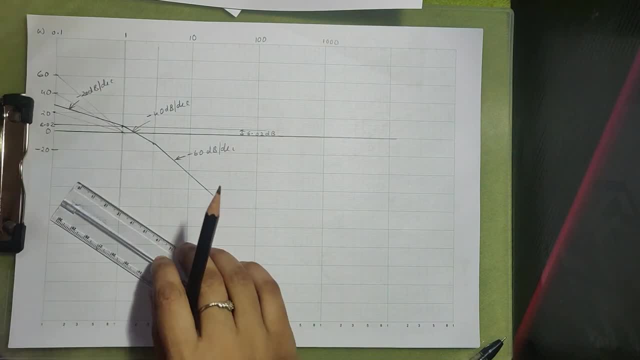 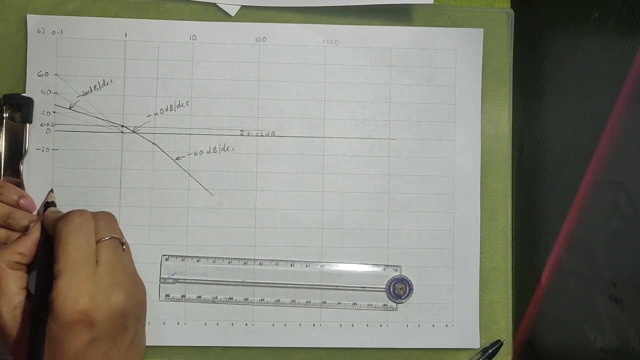 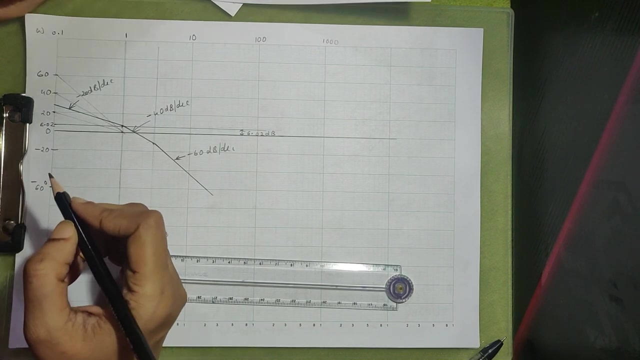 is changing to minus 60 db per decade now. next we need to draw a phase angle. so with phase angle plot we can: okay, i'll just mark here, you can just directly mark here. let it be because in in the phase angle plot we can see all negative angles, so we can put only negative angles here. 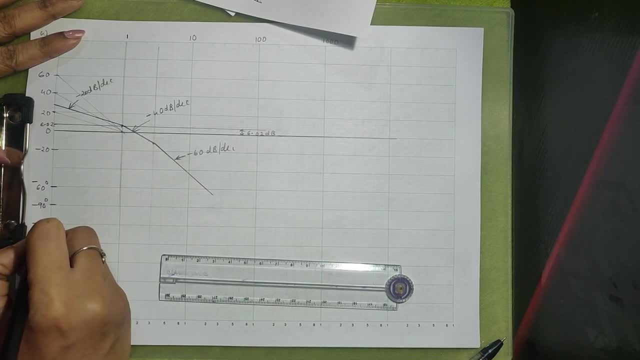 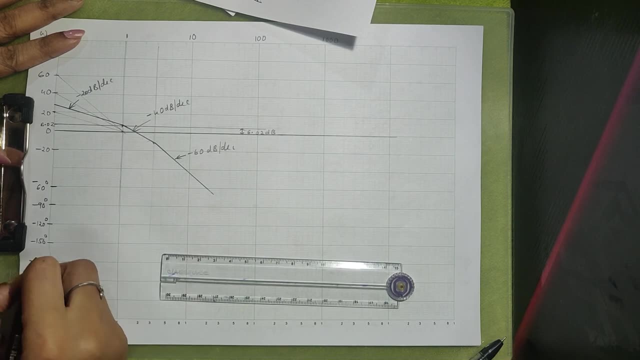 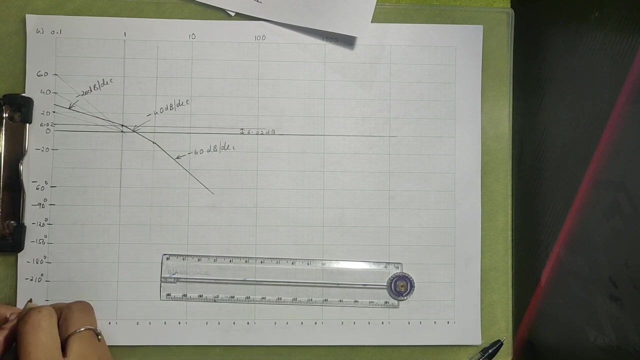 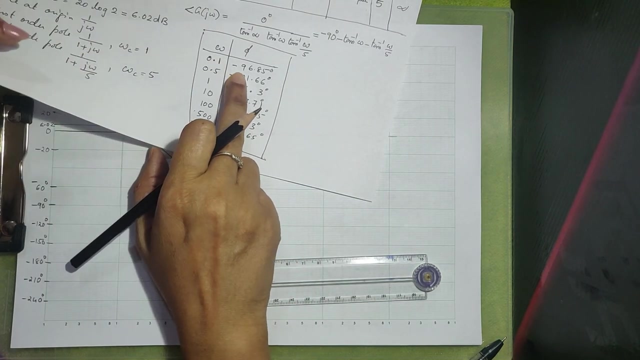 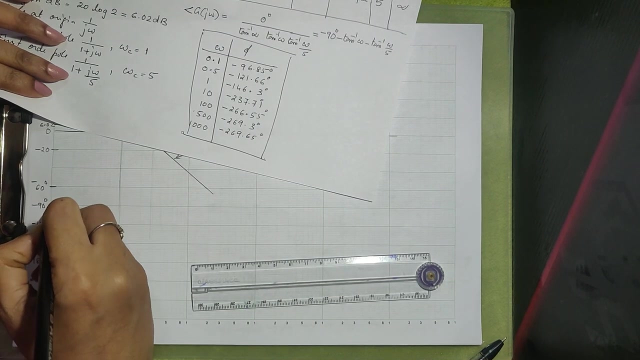 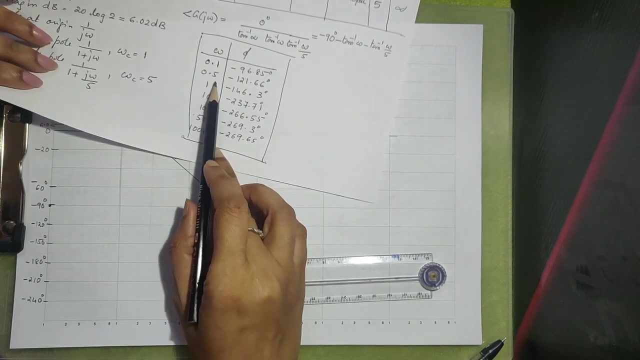 minus 90 degree, so minus 120 degree, then minus 150 degree, minus 180 degree, minus 240 degree. let's see now at: omega is equal to 1. triangle is minus 96.85, 96.85- it will be somewhere here. first point, then 0.5 at 0.5 it is minus 121. 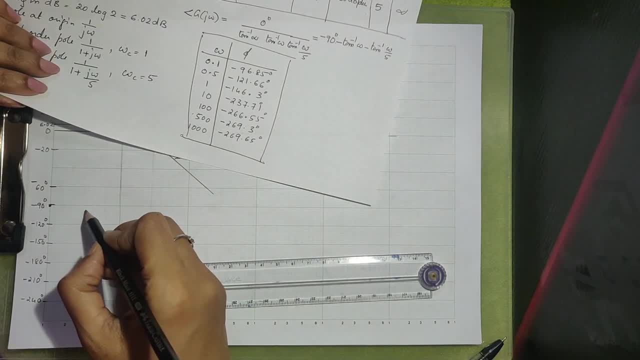 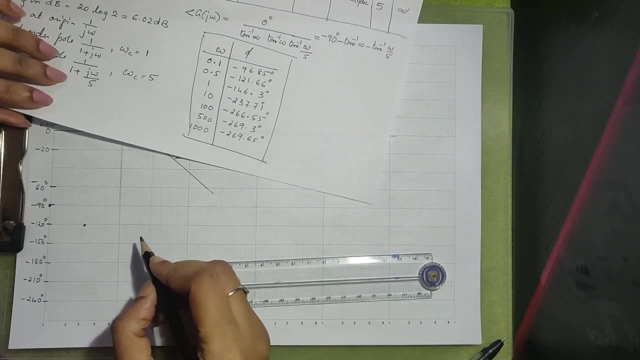 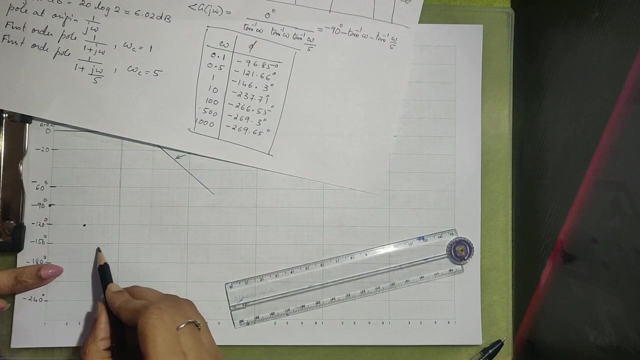 so 0.5, this is. this is the value corresponding to 0.5. it is minus 121. it will be somewhere here. i'm just plotting then: at 1 the value is minus 146. at 1 it is minus 146 120. 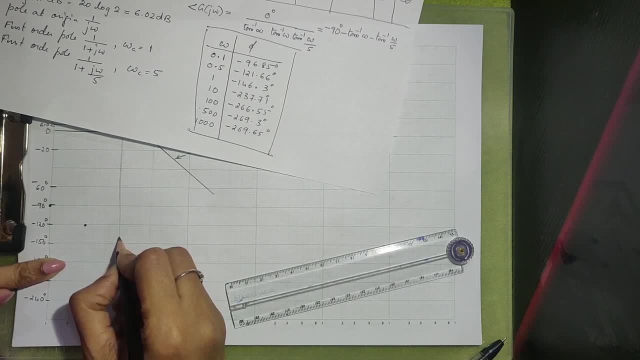 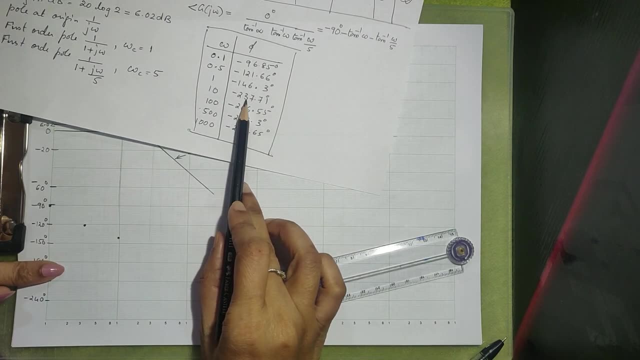 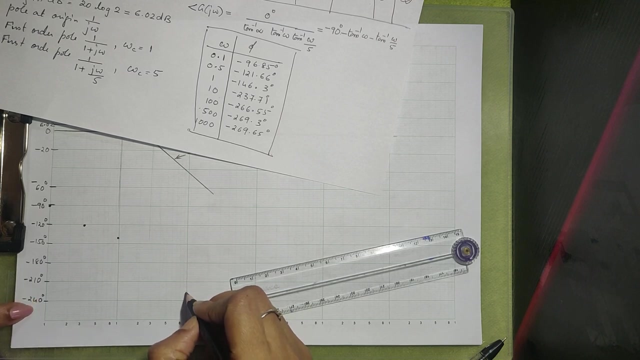 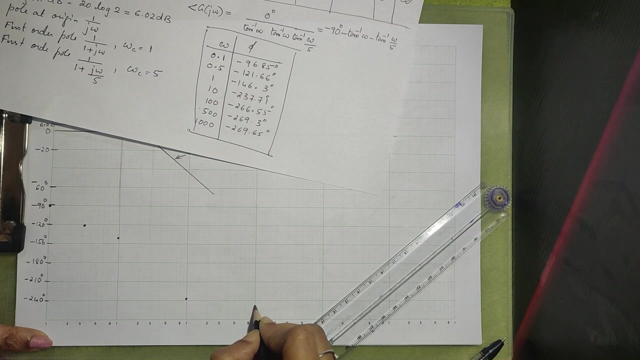 146 may be somewhere here. it is just a rough then. at 1 it is minus 146, 10 it is 237. so this is the value corresponding to 10, it is 237. 237 will be somewhere here. then 500, now 100: it is 266 be somewhere here. 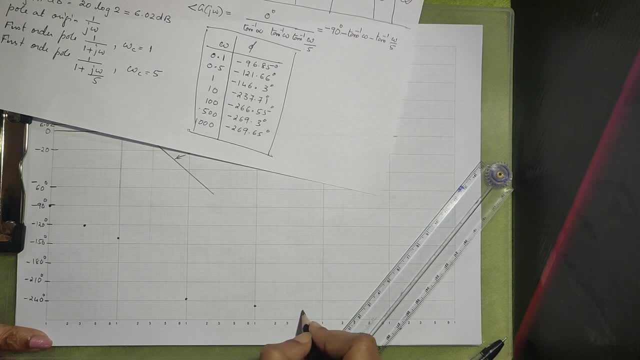 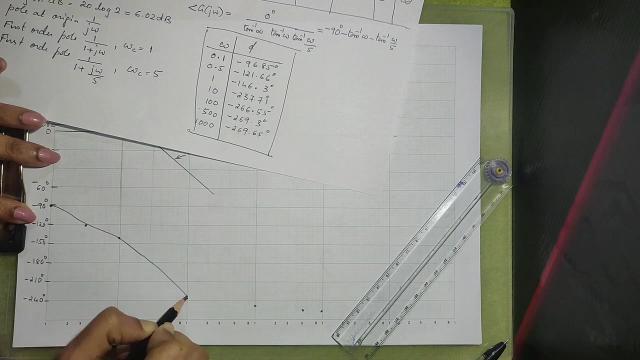 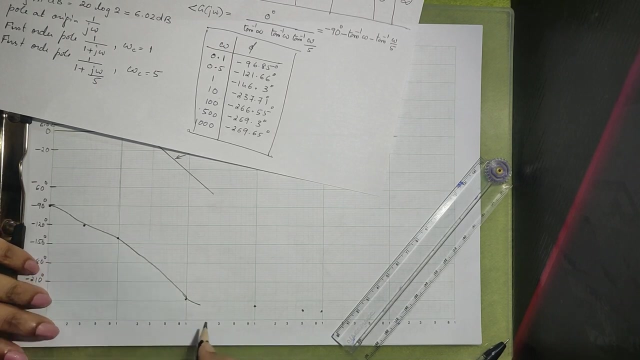 then 500, is here this 269, then 1000. it is again like that. so what we do is we have to actually join this lines, we have to take in between points so you can draw a smooth curve. this one is just an approximate curve, only make sure to take more points. so 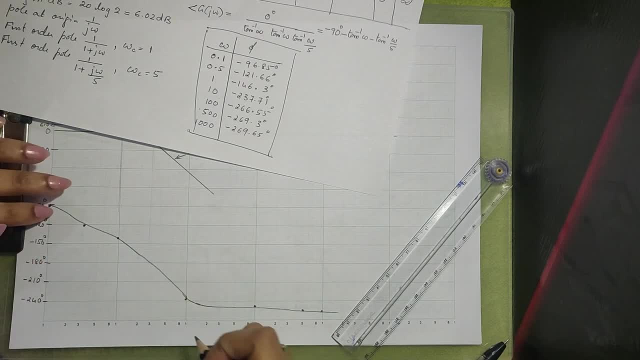 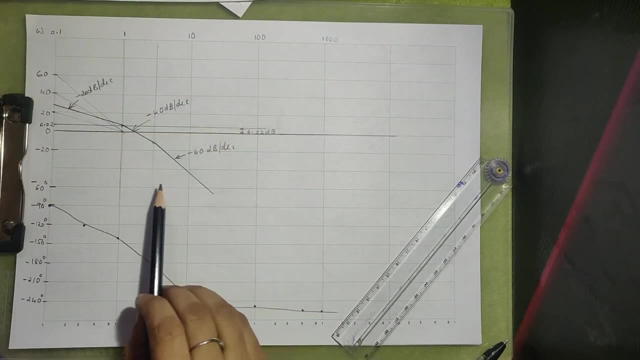 that you will be getting a more accurate diagram now. we have drawn the phase angle also. now what we do is we need to find the margin and phase margin. so how will you find the margin and face margin? so, for finding the margin and face margin, this is found at gain. 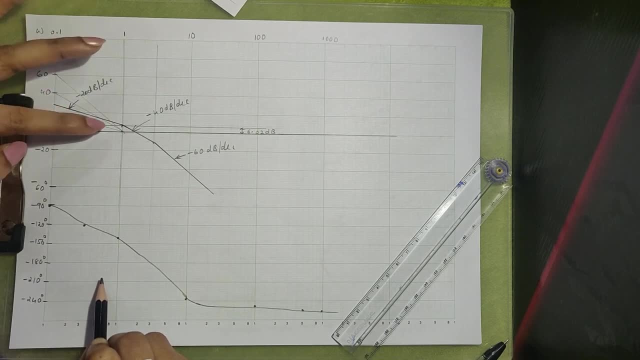 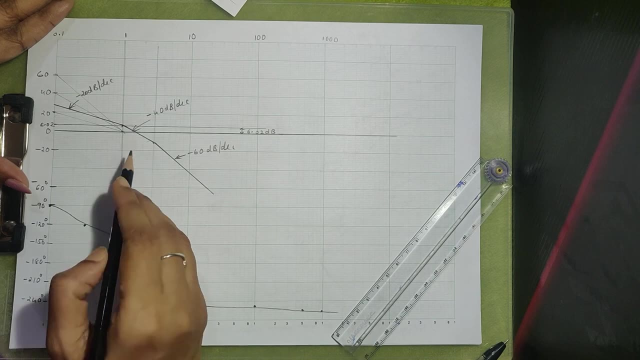 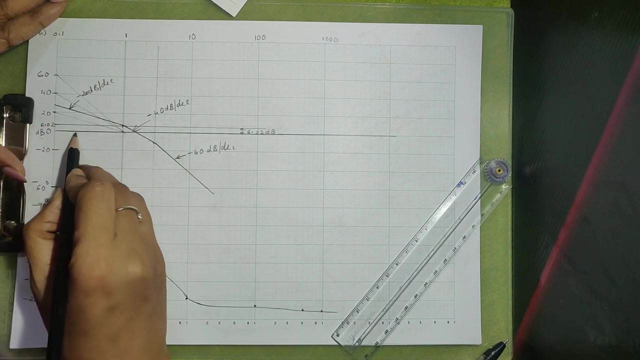 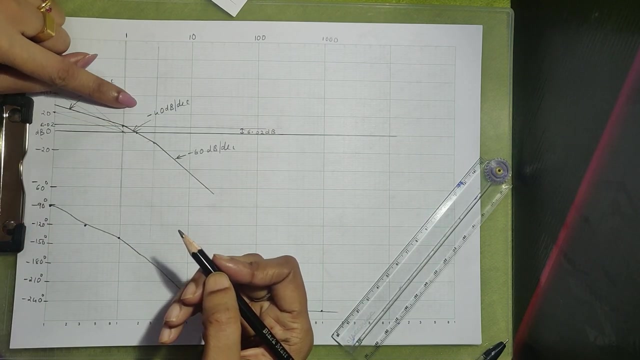 crossover frequency gain. crossover frequency is the frequency at which the magnitude crosses 0 dB line. magnitude becomes 0 dB. so this is the point we can see. this is 0 dB, this is Db. okay, 0 dB, okay. So here, this point: the magnitude is becoming 0, to be find the frequency corresponding to that one. 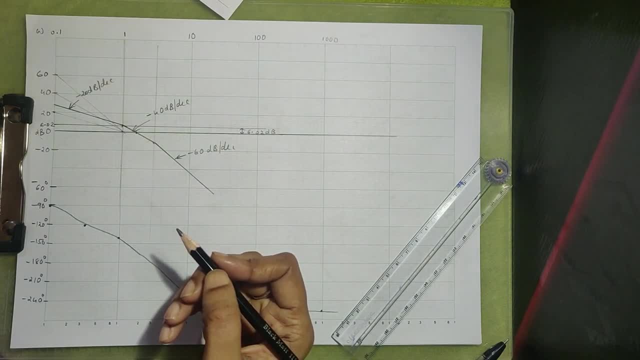 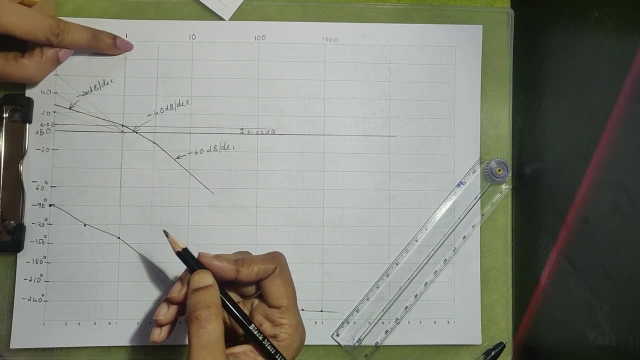 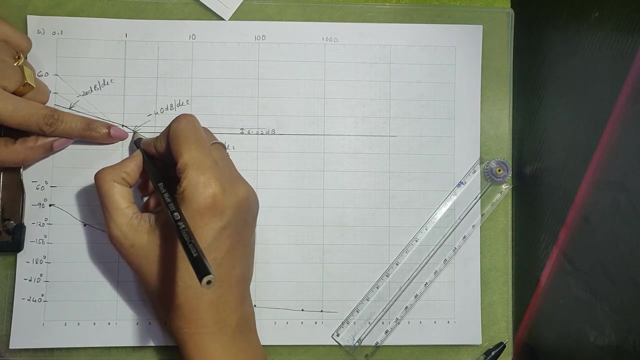 So we will be getting approximately. this is 1.. So we will be getting it as approximately this is the point 2.. So this is 2.. So here it may be approximately. I am just taking: omega gc is 1.4 radians per. 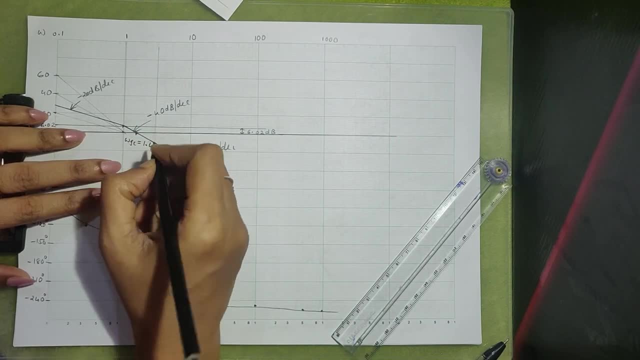 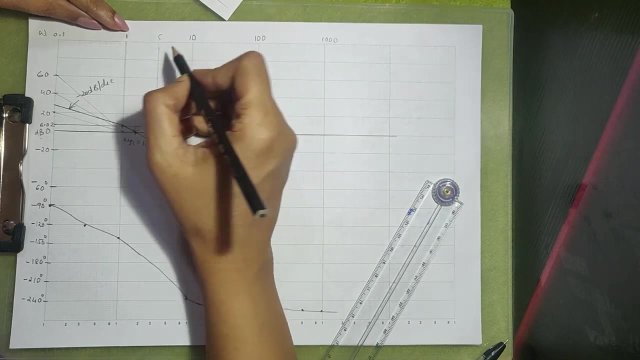 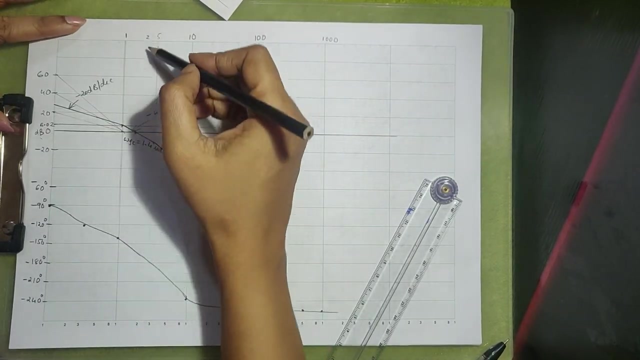 This omega gc is equal to 1.4 radians per second. You take this: this one is 5,, this is 2, this is 2, 5, this, like that you can just see the vertical lines little bit darker. 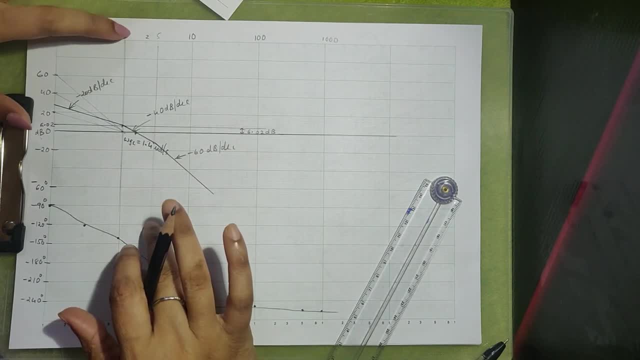 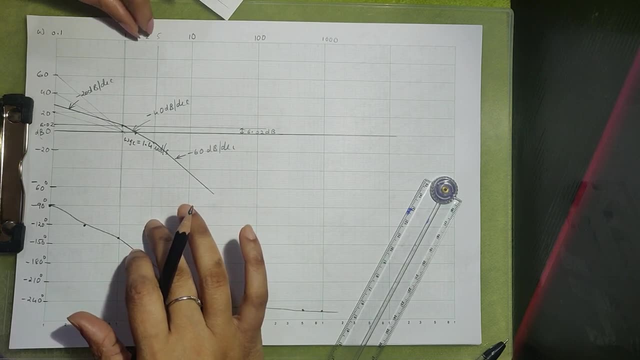 Here. the graph is not the graph sheet. It is not very clear So you cannot identify. So this is 1, 2.. So it is a logarithmic scale. You can see the distance between 1 and 2 is more than the distance between 2 and 3.. 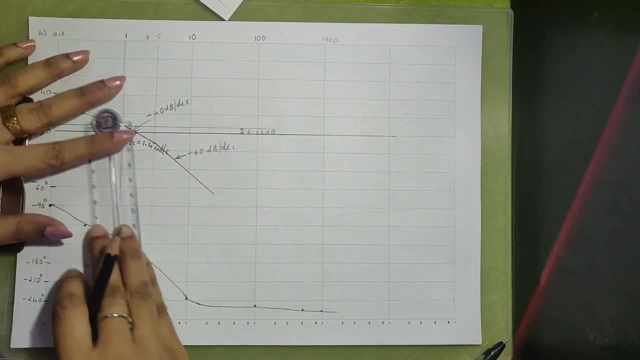 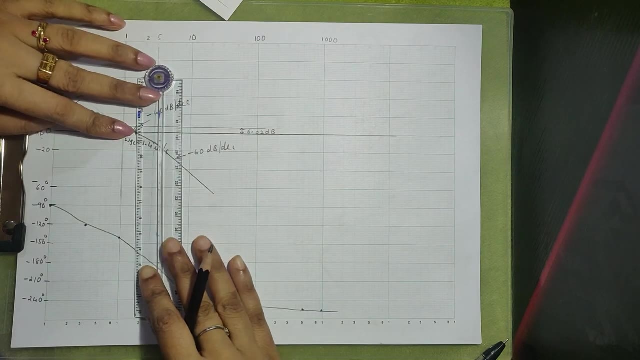 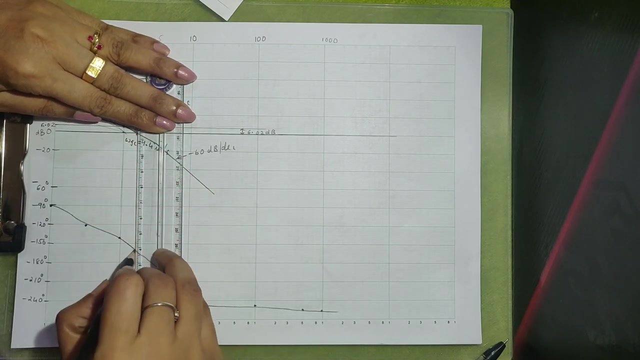 Like that it goes on. So now for finding phase margin. what you have to do is you have to take this point, draw a vertical down so as to cut the phase angle plot. Okay, this one. So this is 1.4 radians per second. 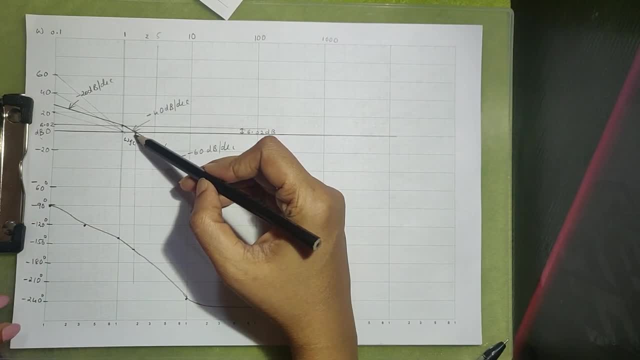 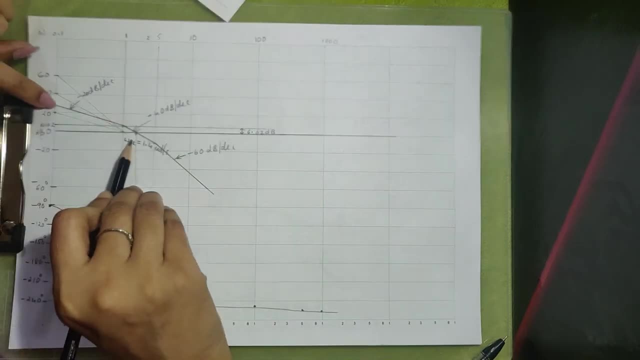 So this is the point where it is intersecting. So what you have done first, you found the gain cross of frequency. Gain cross of frequency is nothing, but it is the frequency at which magnitude becomes 0 dB in our magnitude plot. 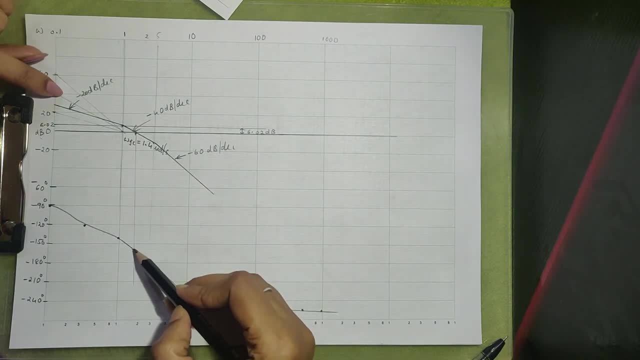 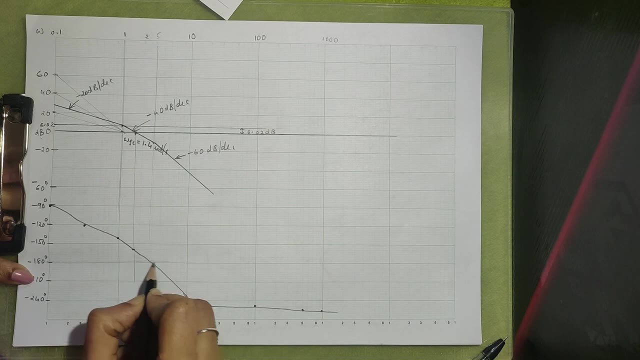 Take that point, bring it, draw a vertical down so as to intersect the phase angle plot. and this is the 180 degree line. 180 degree is this So the distance. this one will give you phase margin, So the value is 180 degree. 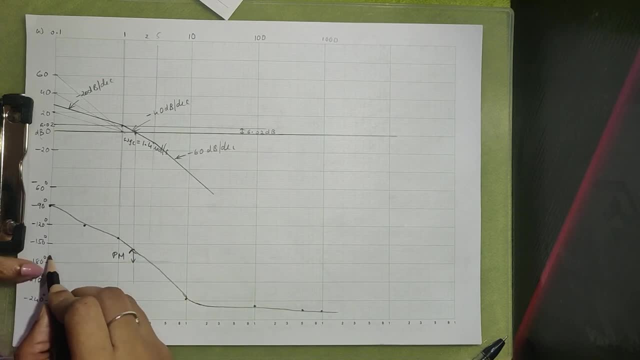 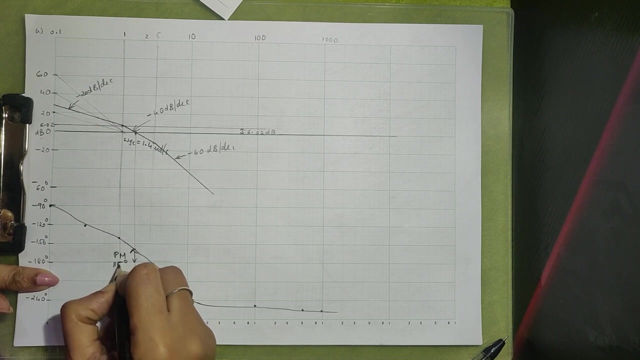 This one 150.. Here it is 150, something It will be coming. So it is that minus 180 degree, plus that one, will be your angle. So phase margin: you will be getting it as 15 degrees, The value this distance will give you phase margin. 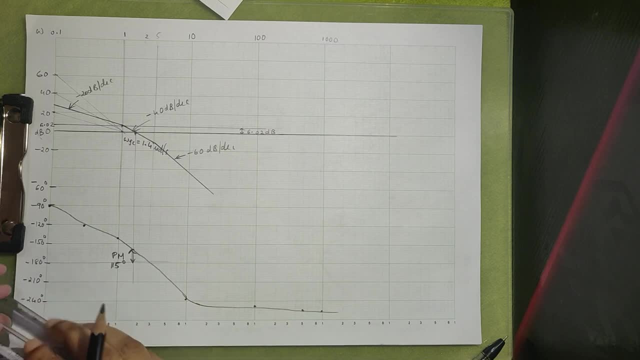 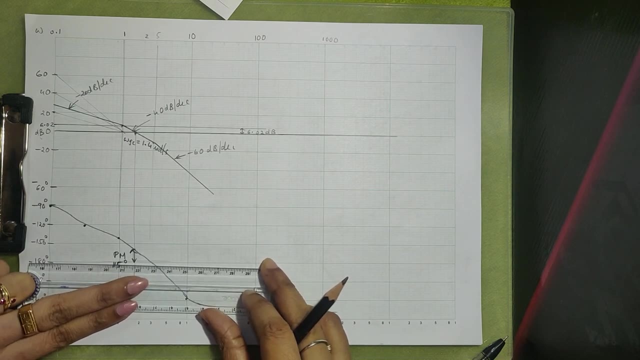 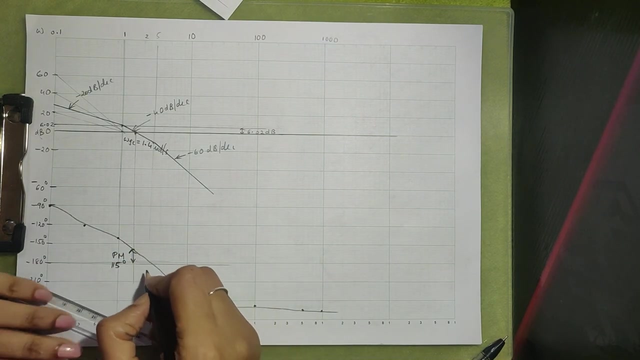 Now for finding gain margin. what you have to do? You take the point 180 degree minus 180 degree where it is intersecting the phase angle. plot this one. So phase cross of frequency is nothing, but it is a point. it is a frequency at which phase angle becomes 180 degree minus 180 degree. 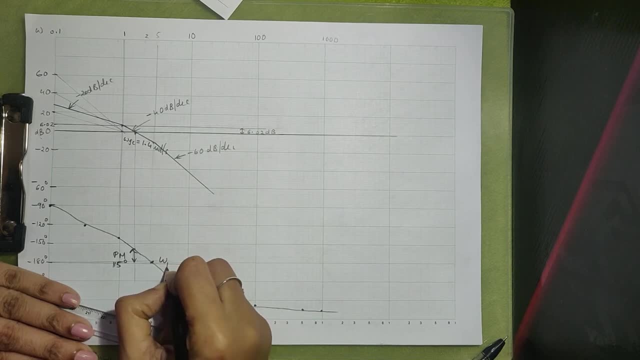 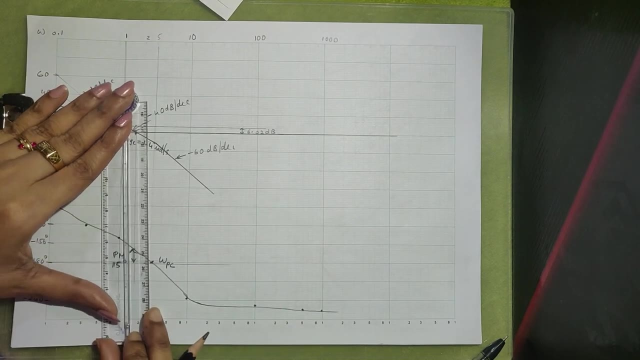 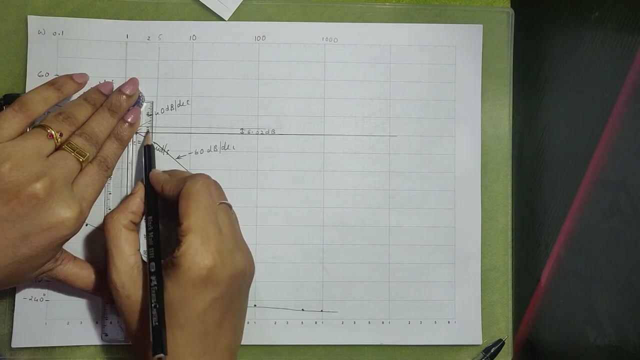 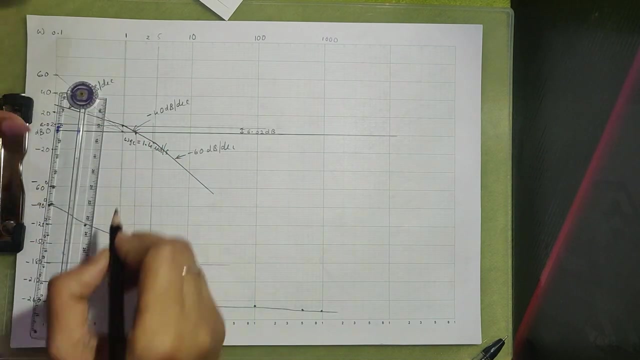 So here you will be getting omega bc phase cross over frequency. Now for finding gain margin: you need to draw vertical up from this point so as to intersect the magnitude plot. Bring, draw a vertical up so as to intersect the magnitude plot. 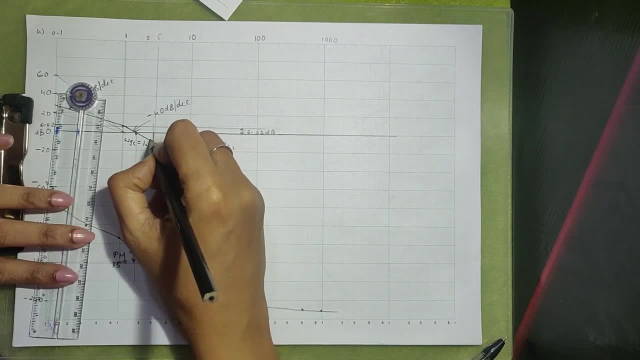 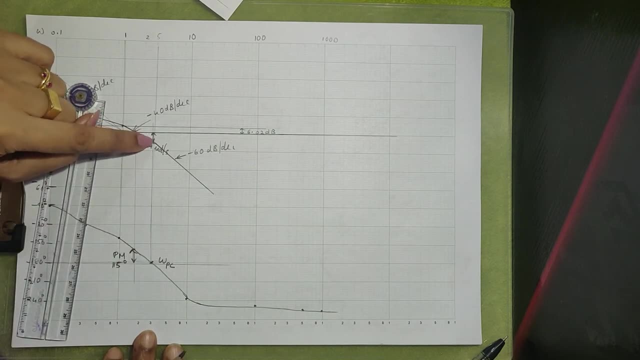 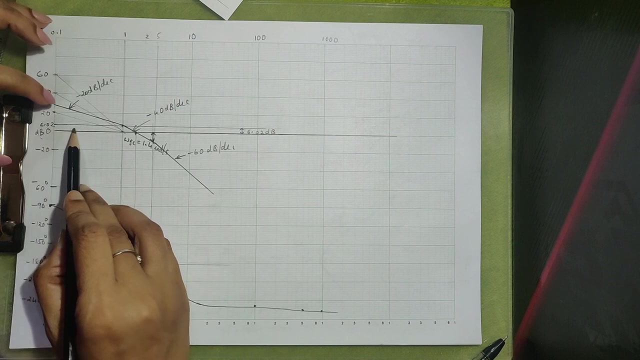 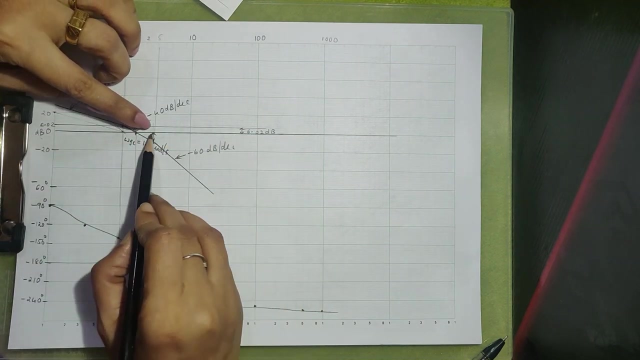 So this is the point we are getting. So this distance. So from phase cross over frequency. you have drawn a vertical so as to So this distance. So this distance, Cut the magnitude plot and the point of intersection of that and the difference between the point of intersection, the magnitude at this and the reference line, that is 0 dB, will give you gain margin. 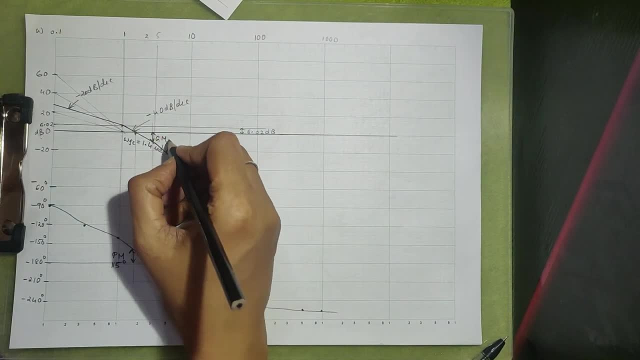 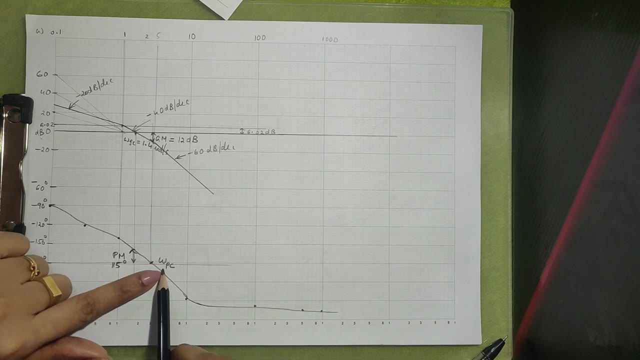 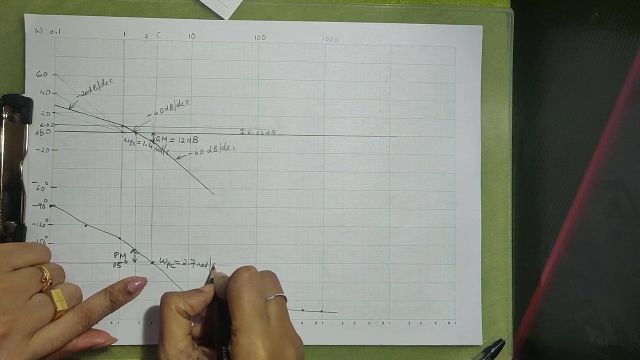 So this distance is actually our gain margin, So gain margin will be getting it as 12 dB. So we got a omega pc. Omega pc is equal to- So that I didn't write it- 2.7 radians per second. 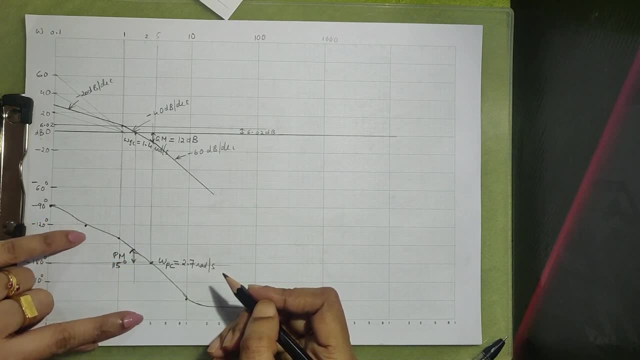 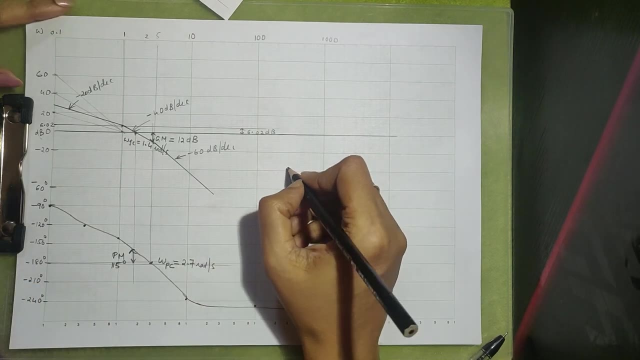 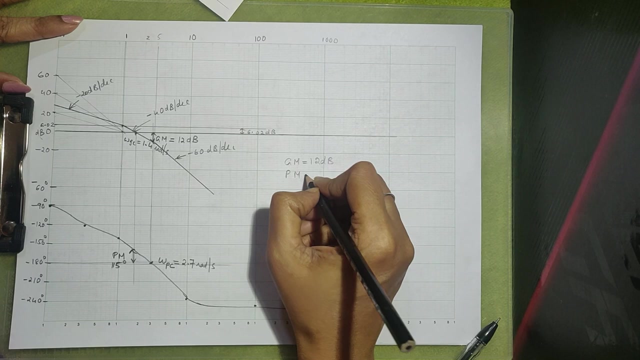 This is 1 point for radians, this is 2.7.. Here you can see, it is 2 point, This is 3 and that is somewhere here it is coming 2.7.. Now you see, here, in this particular problem, gain margin is equal to 12 dB and phase margin is equal to 15 degree. 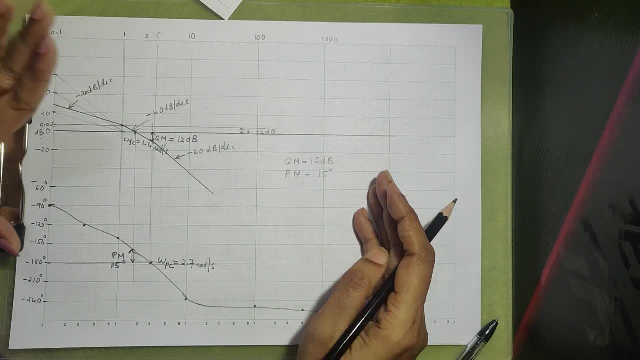 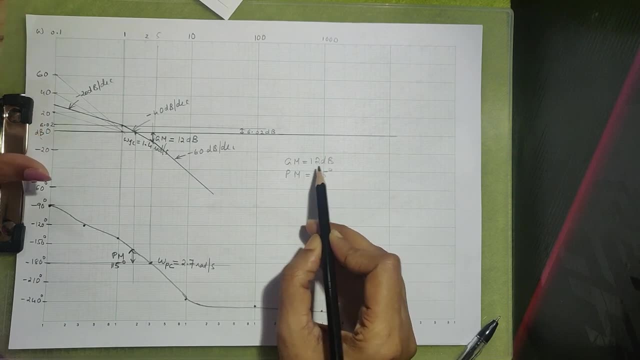 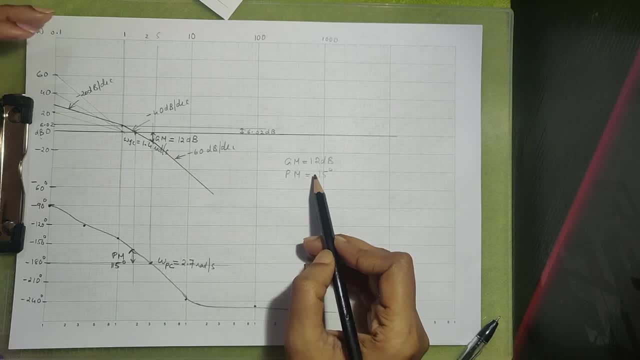 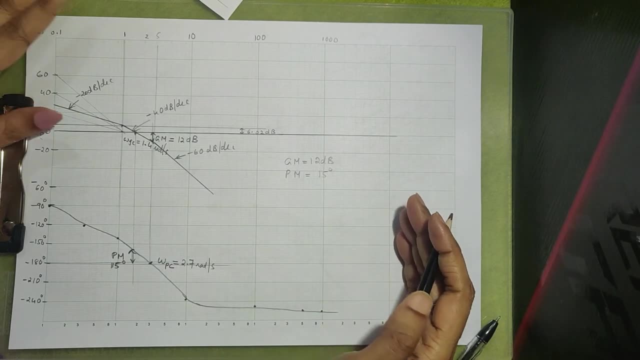 If both are negative means the system is unstable. If both are 0 means the system is marginally stable. So here both are positive. So the given system is stable system. Now, this is how you will be plotting the body plot. 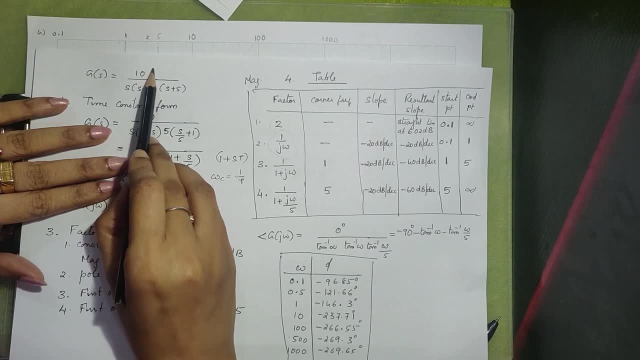 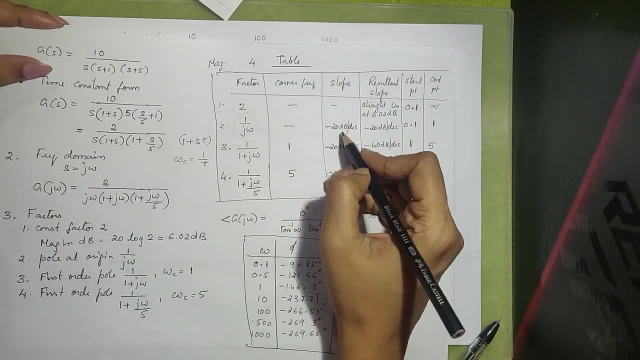 Now one thing I need to tell you. Suppose if there is a 0 present, 0 term present here, Then what will happen When you are forming the table here? The slope becomes here in this one, for first order pole, it will be plus 20 dB per decade. 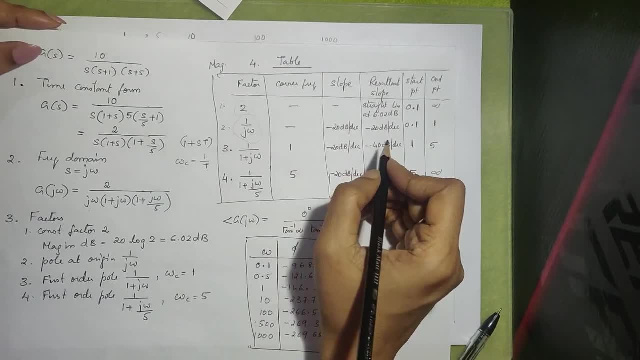 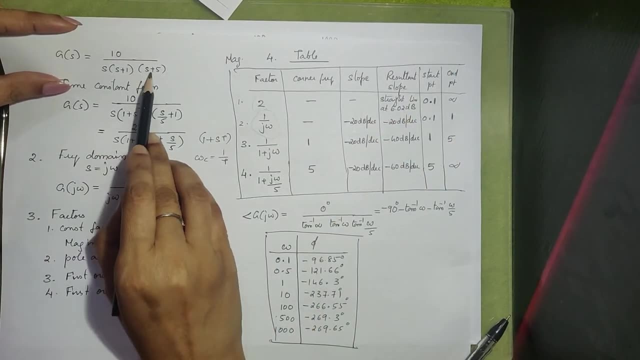 That difference will come, So result, and accordingly it will be changing. So you need to. So, whatever transfer function is given to you, you have to form the table. First you have to put it in time- constant form. Then you have to make it in frequency domain by substituting: s is equal to j, omega. 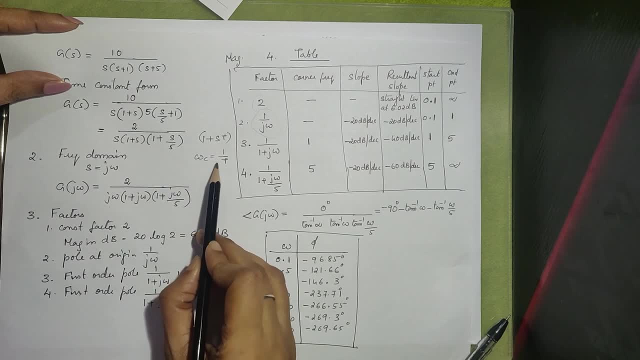 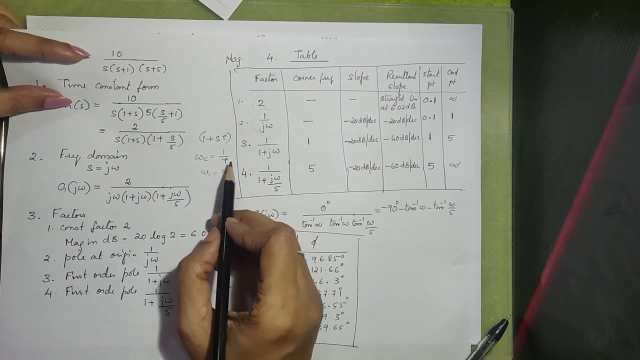 Then find the corner frequencies. For first order factor, corner frequency is 1 by T. For second order factor, corner frequency is 1 by T. For third order factor, the corner frequency is omega n. So once you find the corner frequency, you have to form the table, starting with the constant. 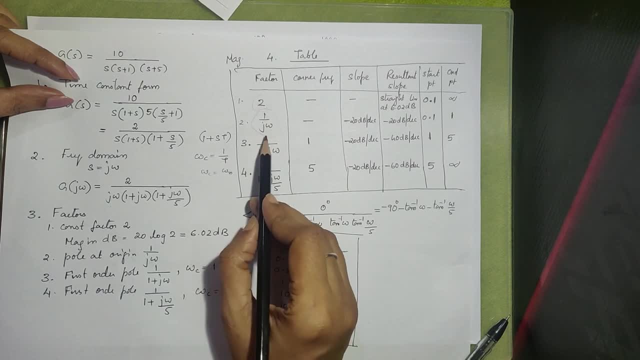 factor and then comes the pole source 0 at origin. Then you have to write the factors in increasing order of corner frequency, So the factor which is having the lowest corner frequency should come first. other than these two terms, If both of them is not present, then you will be starting with the term with the least corner. 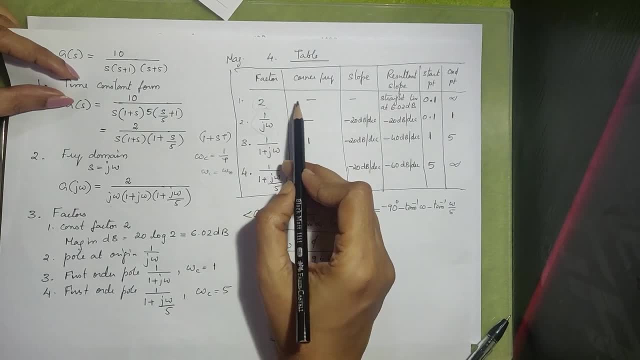 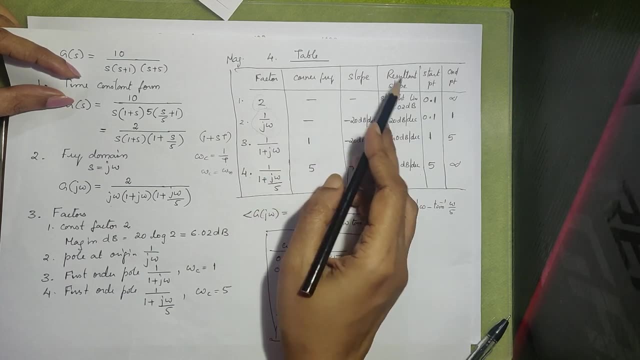 frequency as the starting factor. So if any pole or zero at origin is present in the given transfer function, then that will be the starting slope of the given magnitude plot. Thank you. 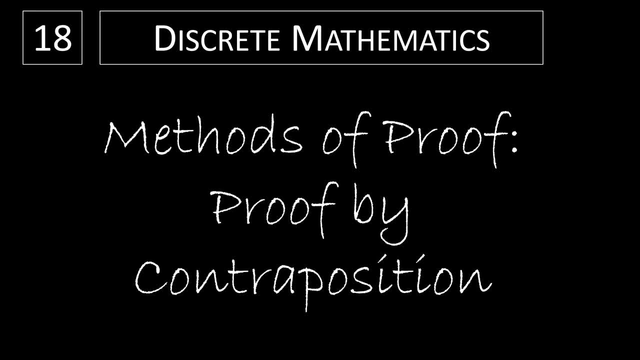 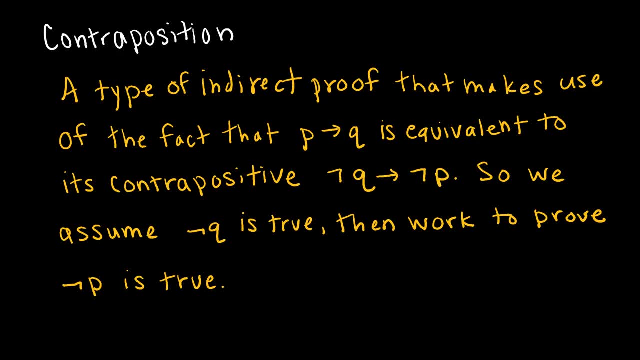 In this video, we are going to look at the method of proof known as proof by contraposition. Contraposition is a type of indirect proof, so we've just learned about direct proofs. This is an indirect proof that makes use of the fact that we